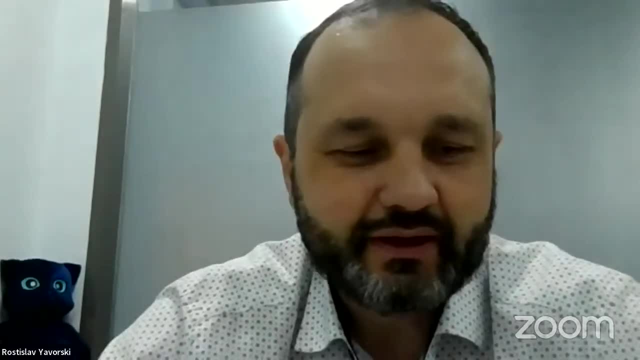 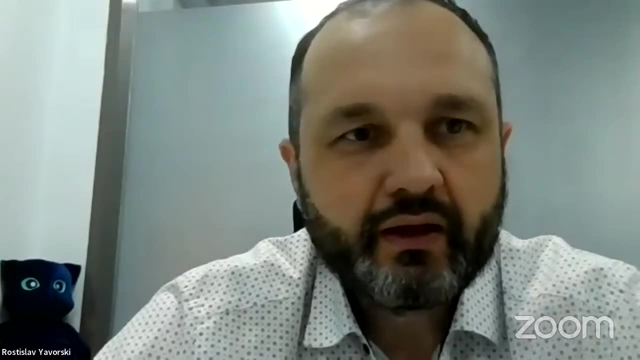 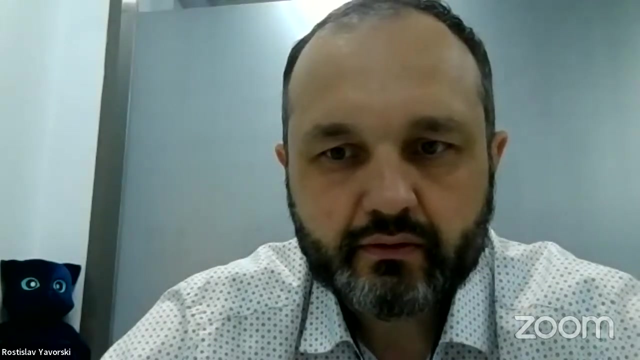 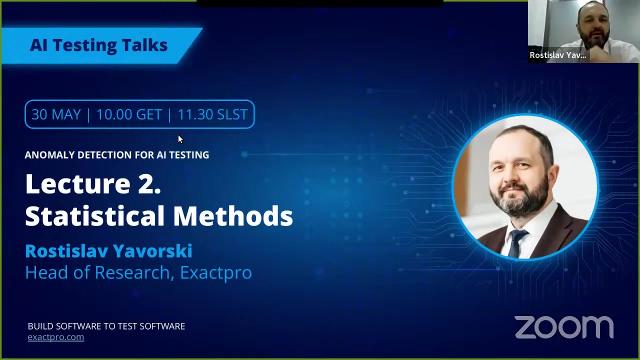 previous lecture number one, which was mostly very introductory, about numerous examples why anomaly and outlier detection is very important, And today we'll speak about statistical methods. So let me share my screen. Okay, you should be able to see my screen. So lecture number two. 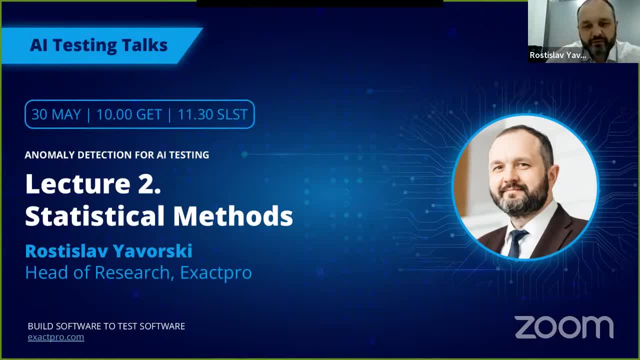 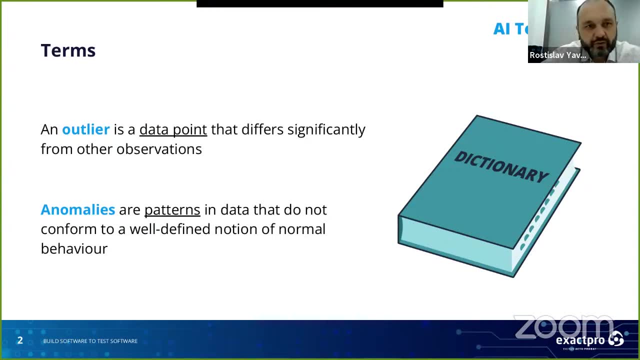 anomaly detection for AI testing, and we'll speak about statistical methods. So let me start from reminding you some of the most basic terms of our course. So outlier is just a data point that differs significantly from other observations. And again, just let me repeat again: 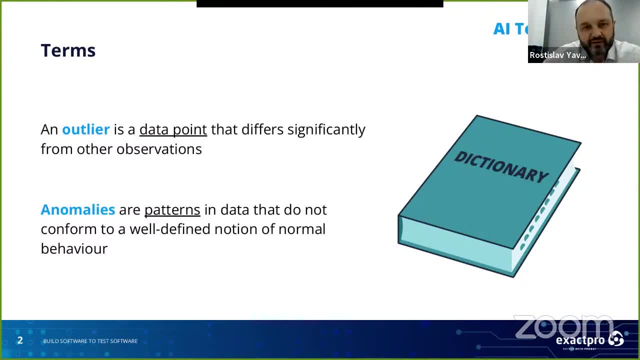 and again that this is not a formal definition, because significantly is not something you can easily formalize. The second definition is slightly more wide, So sometimes we're not looking for just one data point, but maybe for some patterns, And we use the term anomaly. 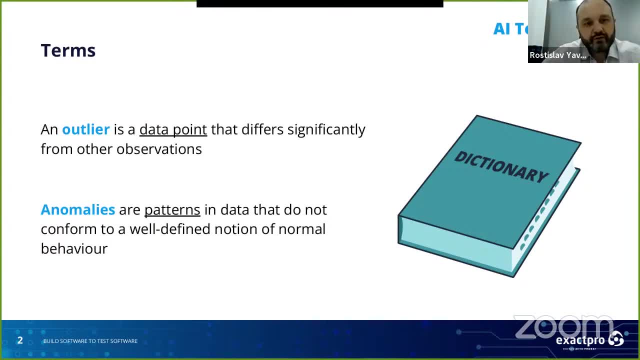 although these terms are interchangeable, Usually we use the term anomaly for patterns in data that do not conform to a well-defined notion of normal behavior. Again, before defining abnormal, you need to know what's normal, and that's not really easy, And we will speak about it again and again. So this is the plan for today. We start with very 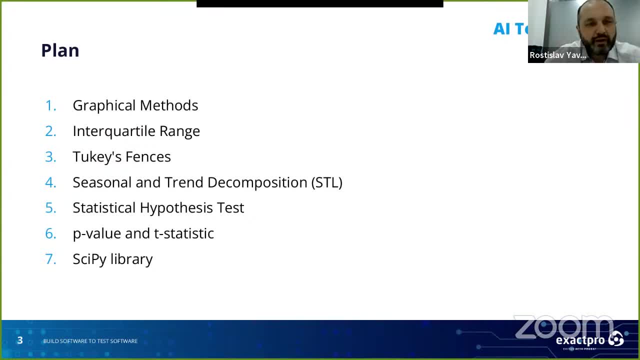 simple graphical methods and very basic notion of interquartile range, And then, gradually, the technique will be more and more advanced And we'll finally speak about statistical hypothesis tests and p-value and t-statistics, etc. So let's start. 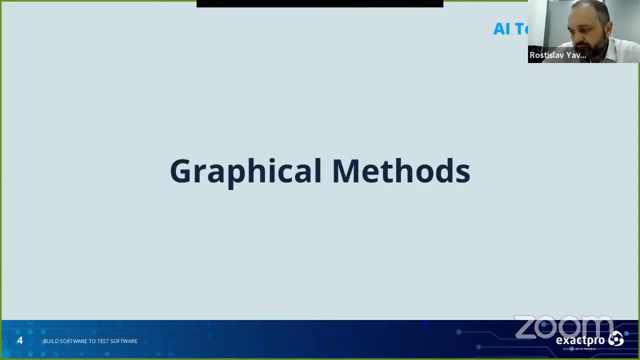 Our main goal during this course is to figure out how to detect anomaly, And usually the simplest approach is just to visualize your data. So once you have a picture just in front of you, then you can easily figure out that, okay, this could be probably anomaly and this could be. 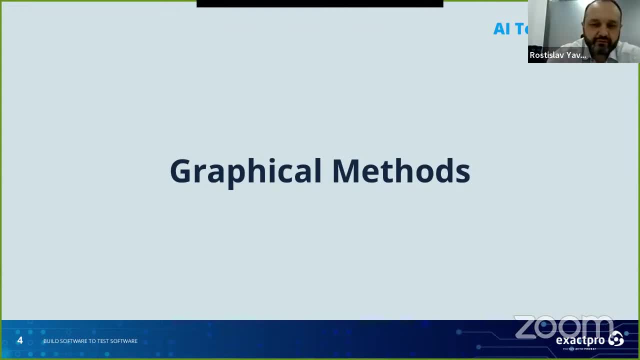 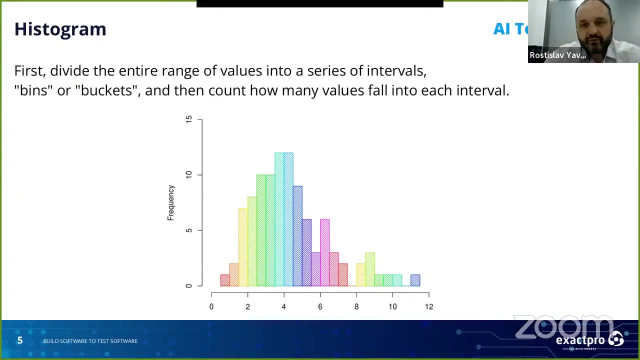 outlier. So the first method is just to build a graph, And the histogram is probably the simplest solution. So for those who are not maybe very good in this, let me remind the definition. So you just divide the entire range of your values into several intervals, which are called bins. 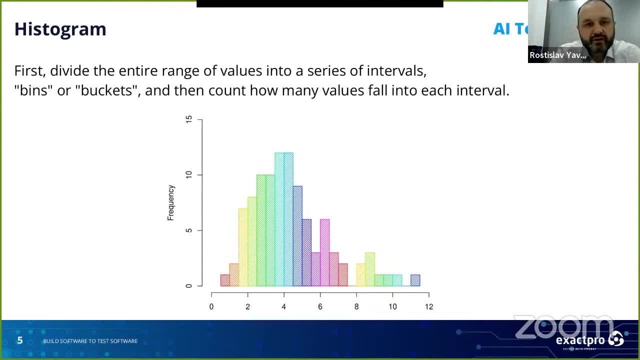 sometimes buckets, And then you just cut out how many values fall into each interval. So here you call this: each bucket is colored in different color. Okay, this is probably nice for the lecture, but usually people don't do it this way. But anyway, you can easily see that values around four are quite frequent. then some values. 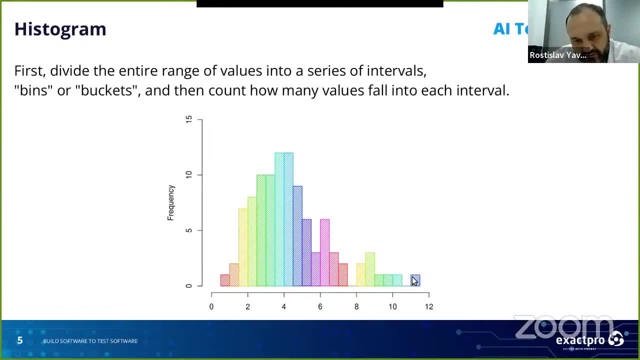 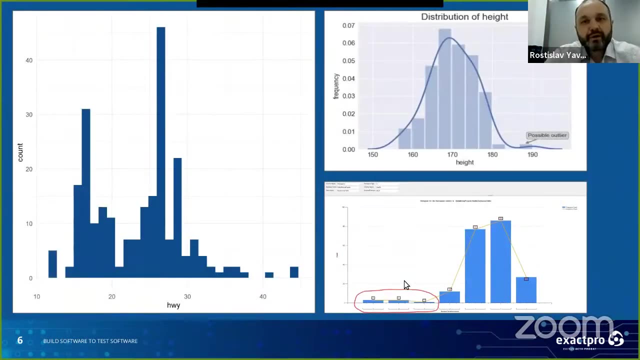 are not And the value you see in your data set you have a value which is close to 12. It's here and that looks quite like not really normal, So that could be possibly an anomaly or outlier. So here are more practical examples from real life And you see that 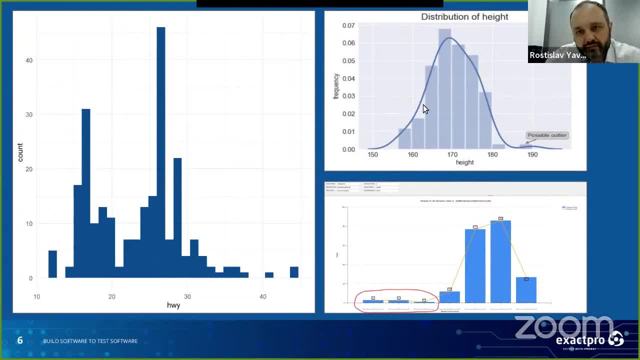 sometimes your graph could be unimodal. So you have just one interval with most data which are here, And then you see here some possible outliers. It's easily seen from the picture that it could be somewhere here. This is another example where 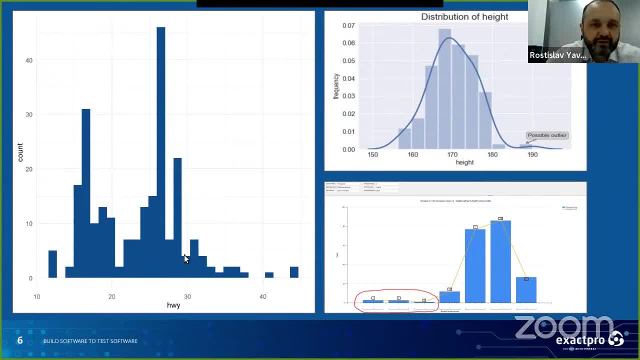 you clearly see that you have at least two different groups of data, which is probably this different distribution. So that's not that simple to analyze. But anyway, even from this graph you see that there are some values which are far from kind of standard. 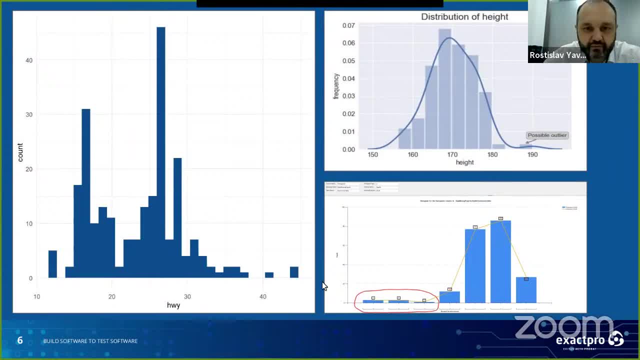 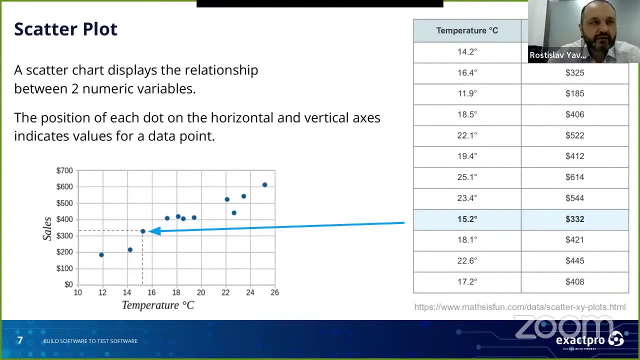 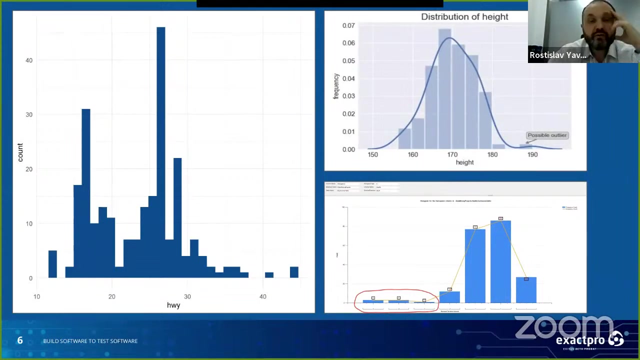 And again that could be kind of candidates for outliers or anomalies, And this is another example, So anomalies here on the left. Another very useful and very important technique is Cutter Plot, So what's kind of a big part of Histogram. So with Histogram you can only 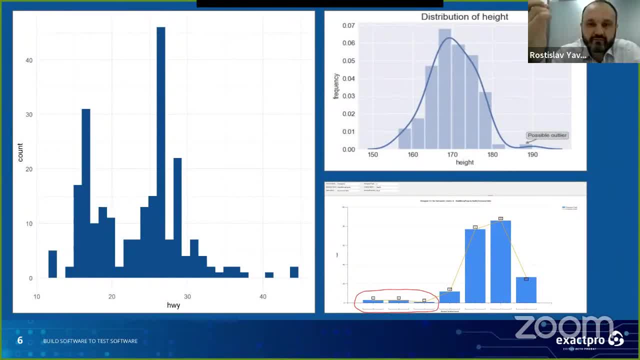 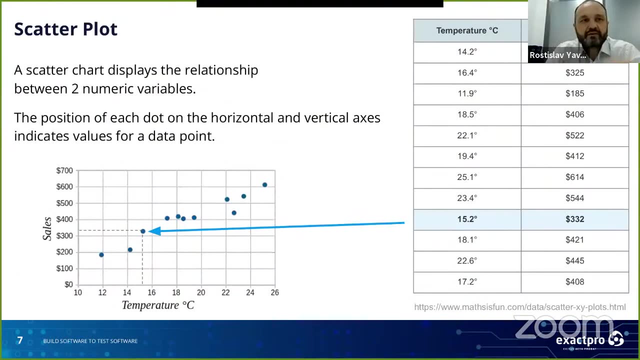 realize only one parameter. So you have like some hate or weight or something else. You just count, So you visualize how this parameter is distributed. but usually your data has much more than one parameter And Scatter Plot is a technique which allows you to realize two parameters, For example. look at this picture on the right: 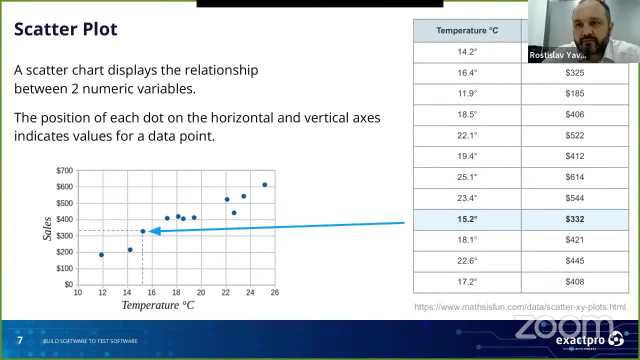 You have some data which describe ice cream sales depending on average day temperature. So you measure some like your weather parameter, like 16 degrees, 22 degrees, I think, Celsius, And then you sell so many ice cream So you have some income generated like 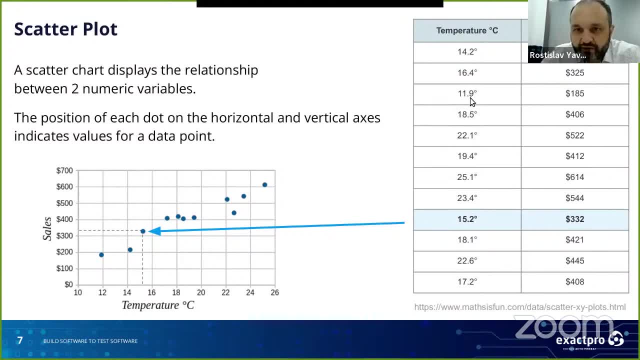 $100 or maybe $500.. And you definitely see, when the weather is cold, then your income is smaller. When the weather is hot, then definitely you sell more ice cream. So again, the technique is quite simple: You use one axis for temperature, another one for sales. 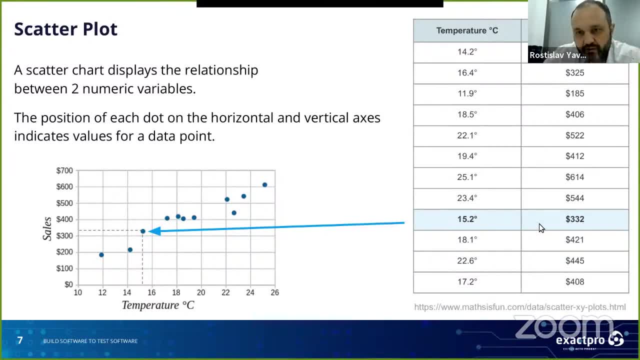 Then each particular data item. here it has two parameters like this one: 15.2 is somewhere here, right, Yes, And 332 is somewhere here, So this point corresponds to this data item. So this technique is much more powerful, because you can visualize a relation between: 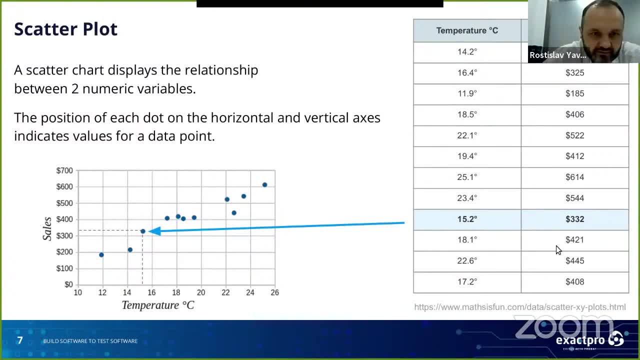 two different parameters. And again, part of this picture is that the order is not visible here. For example, it may happen that the order is important for you, That this was the first day, second, etc. But here on the picture, 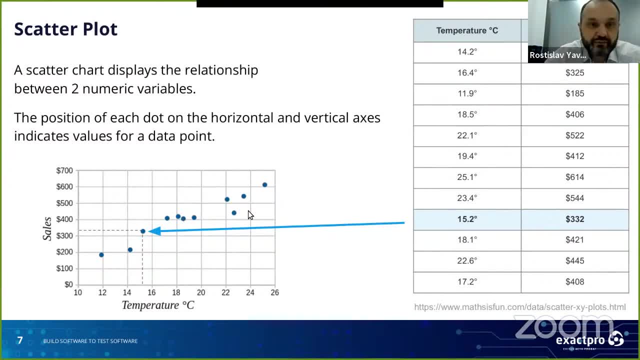 the order kind of is lost. So you just have the set of this point. It doesn't matter which order. No, no, It does matter. But it doesn't matter either. But youmind, if they are here And they're not. No, These are the three Fuck-and-clock points right now, right Like because the order becomes smaller. So what are they going to be related to here? And you can spend a lot more on this at the end of the story, But again, the big part of this picture is that the order is not visible. here, For example, it might happen. 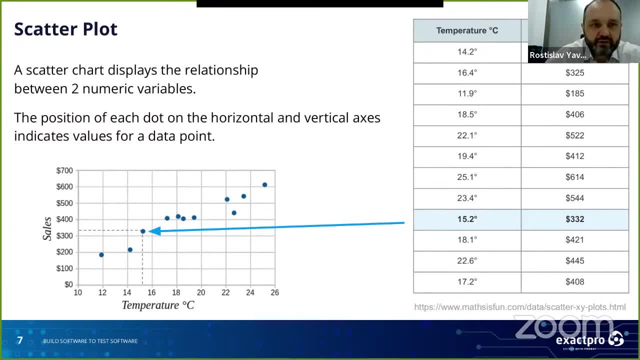 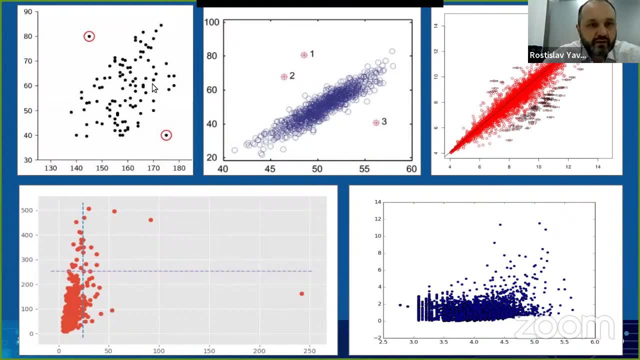 but you cannot see it on the picture. so in which order they are up? So here are some examples from real life and you see, sometimes it's quite easy to figure out that these two points probably are candidates for outliers. Sometimes, yes, we have like this one. 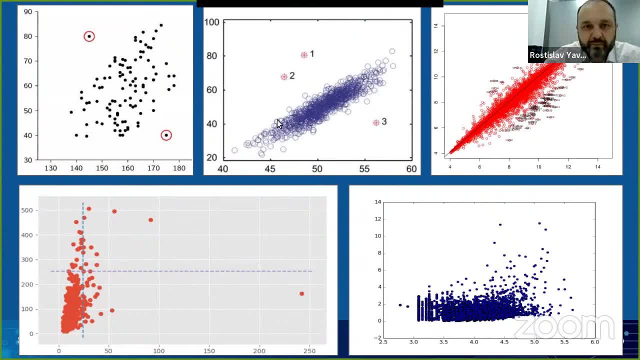 so you may have quite many data points so you can use not points but circles just to see the more dense area, etc. Sometimes you have some kind of pattern, a linear or like here, maybe something more complicated. So you see, sometimes it's quite. 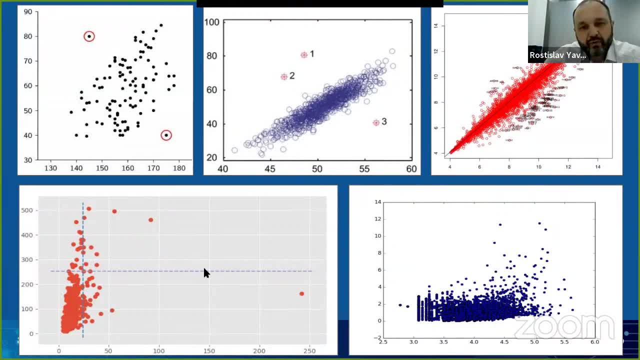 simple to analyze this kind of picture. but more often, the picture does say something to you. but again, it relates to the data. It relies on your intuition, on your experience, whether you can see if, okay, this definitely looks like an outlier and this probably too. but if you speak about these two points, 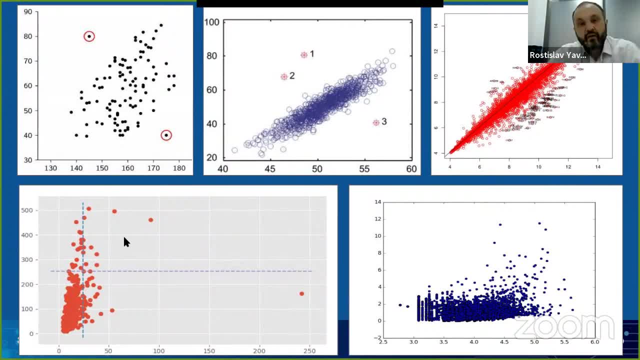 I'm not sure because, again, it depends on your domain. Sometimes it could be, sometimes it's not, but this is a very useful technique. I really recommend you to use it Right. so what's the question? So what's good about this technique is that you can actually see the data. 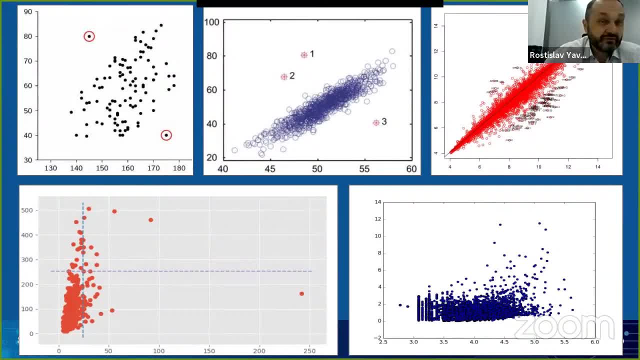 and sometimes it's very useful, but sometimes it's not. For example, you need to design some automatic tool which will check, like maybe even simple test of outliers, and automatically produce this list of candidates and send it to your auto manager. Then involving a human is not. 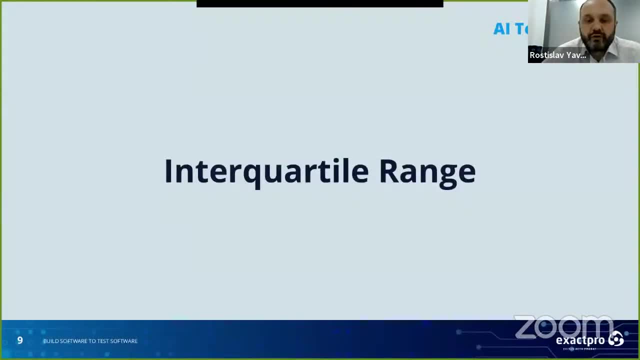 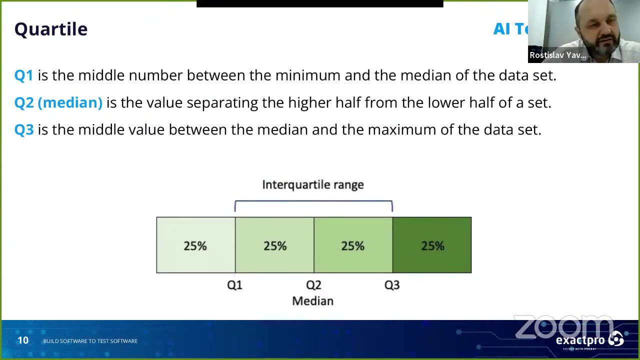 a good choice here. so you need some formula, And probably the simplest formula to detect outlier or anomaly is interquartile range, and let me speak about this one. So again, still very simple, but very powerful definition from statistics: the definition of quartile. So there are three quartiles for every. 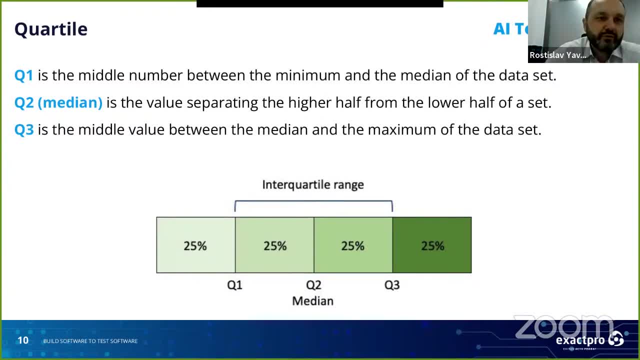 data set and here are kind of more informal definitions. So Q2,, which is second quartile, is already known to everyone as media. So it's the value separating the higher half from the lower half of the set. Then actually you find median. 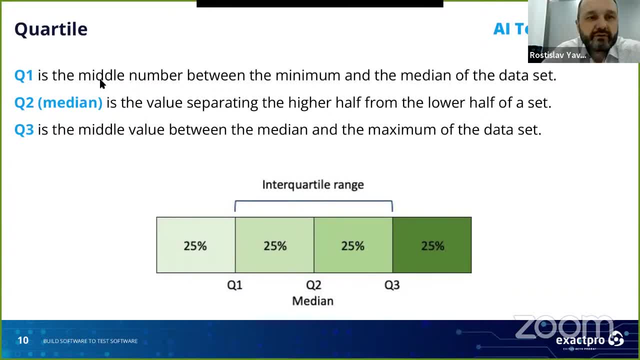 inside the lower half and it's called the first quartile. So it's the middle number between the minimum and the median of the data set. And similarly, the third quartile is the middle value between the median and the maximum of the data set. So, because this is a really important 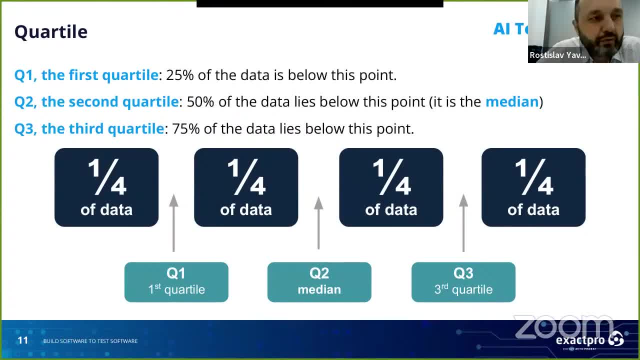 notion. let me maybe spend a couple of minutes more on this definition. So once you got this, Q1, it means that 25% of the data per quarter of your data is exactly. one quarter is just below this number. So Q2 is the value, such that 50% of the data lies below this. 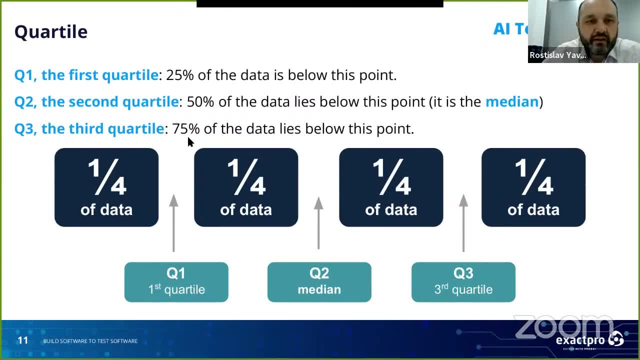 point and another 50 is above. Then third quartile is a point such that 75% of the data lies below this point. So first one, second one and third one. So usually people don't use term. second, because median is kind of more. 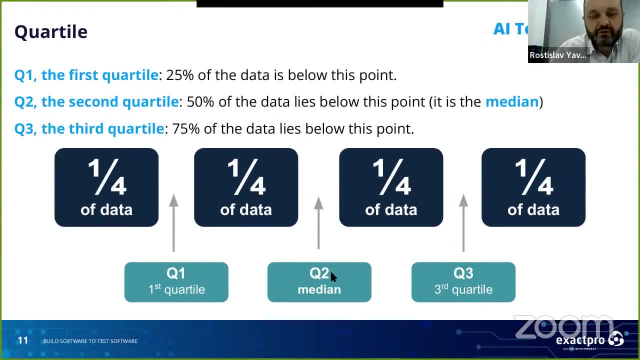 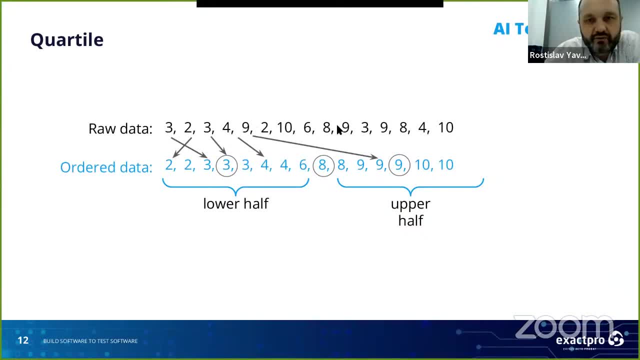 typical term, but actually median is the same as second quartile. So let's consider the following example: Like you have raw data like three, two, three, four, nine, two, ten, I don't know what could be just anything. so you just have some measurements. 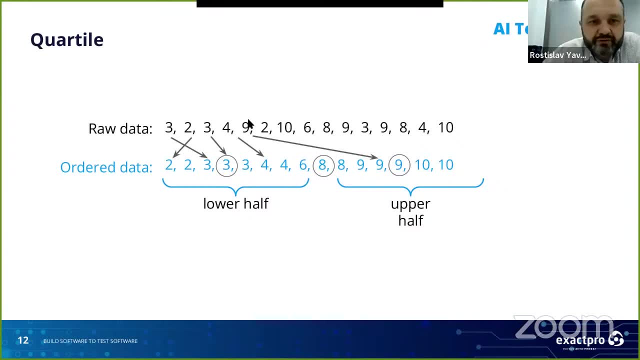 So, in order to compute your quartiles, you first need to order the values Like you see: the smallest one goes here, two, then you have another occurrence of two, then it goes here, then you have three from here, another three from here. 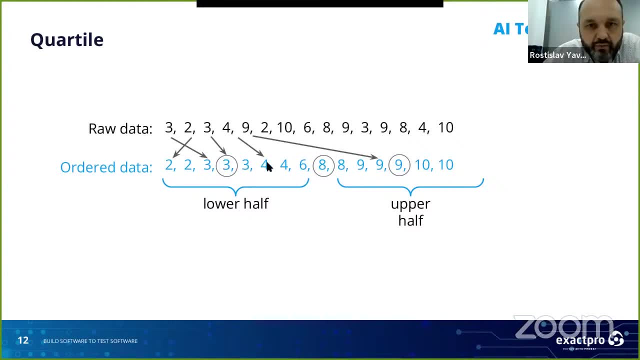 yes, this is another three. it goes here. then you have four, here's another four and six. So a very simple procedure. So the idea of this technique that you can easily implement it manually using any script or programming language. so it's quite simple and doesn't require any. 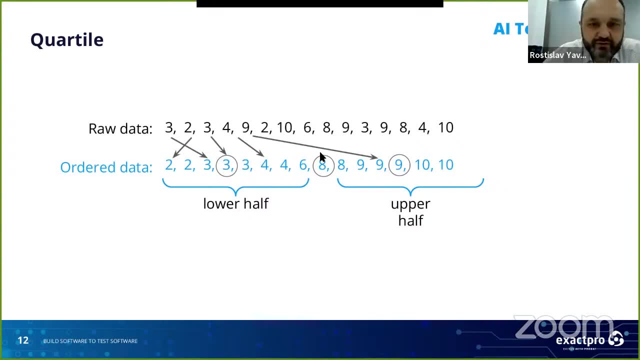 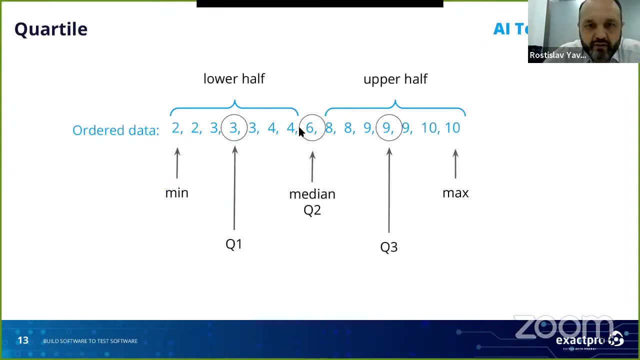 advanced mathematics. So once you order the data, then it's immediately you got the quartiles. So here eight, sorry, six is the median, because it lies exactly in the middle. So then you have minimum, it's clearly two. then you have maximum, it's clearly ten. and then 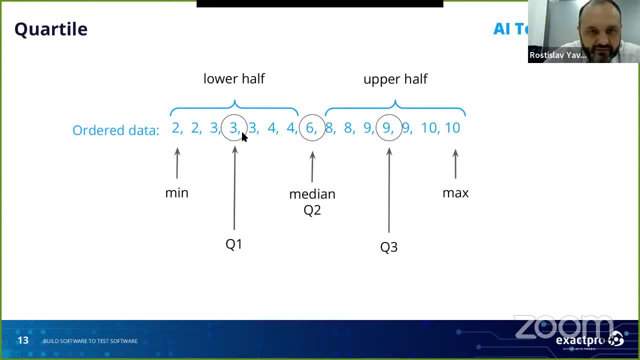 first quartile is the value just in the middle. So you see, three below three items is above, and this is the lower half And the similar way upper half. you have three numbers above, three numbers below. So here you have two. three is the third quartile. 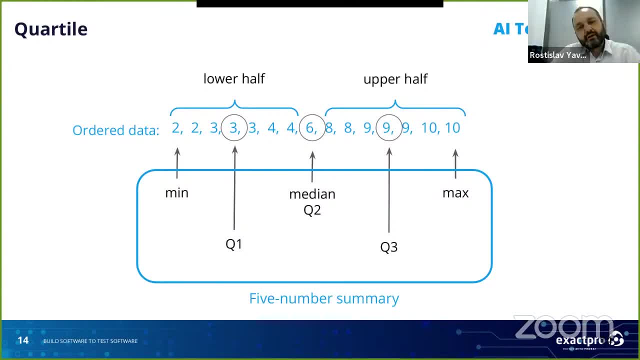 So what's really also very useful and very important from this technique is this is a called five number summary, So typically we don't have much time to communicate our insights from data analysis, For example. you've got some data, you are an analyst and you're speaking to. 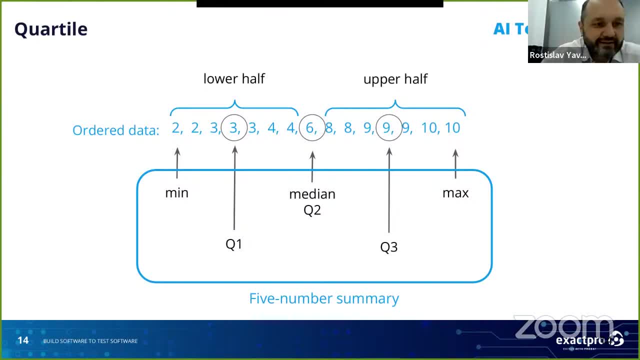 some colleague, friend or manager and he or she is asking you: okay, tell me just a couple of words about this data, And if you're really short of time, just say maybe one word: Okay, the average value is like 22.. Okay, so that's it. Okay, let's move on to the next one. Okay, let's move on to. 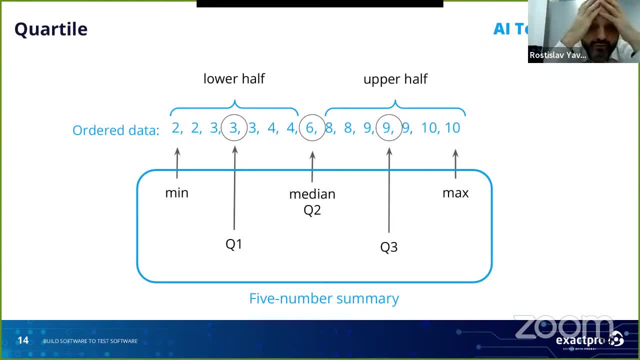 the next one. Okay, let's move on to the next one. So our sales, for example, annual sales, are around like 52 something And this is kind of one number summary, But sometimes you need to add more information and use three number summaries. You can say minimum, maximum and some average or 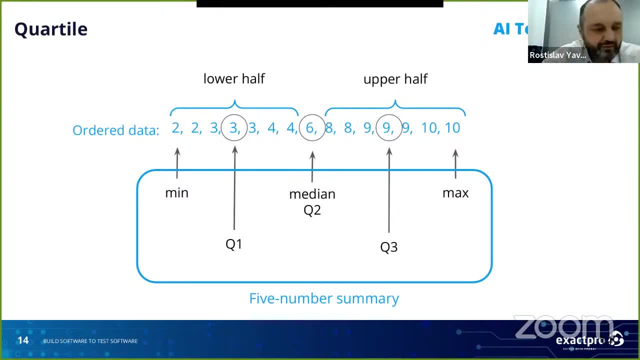 median value. You say, okay, like our daily sales or weekly or whatever is 22,, but the minimum is like 19. So it's never below 19. And the maximum is like 32.. So we do have some value, 32, in our data. 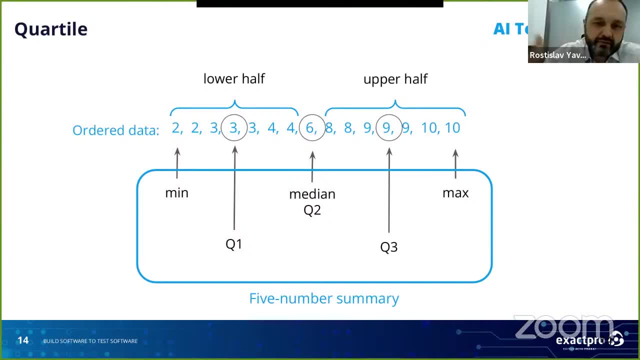 set. The minimum value is never below 19,. but the average number is 22.. So this is already much, much more information. So it already gives you expression that actually you understand. you have more kind of feeling, intuition about the data set And 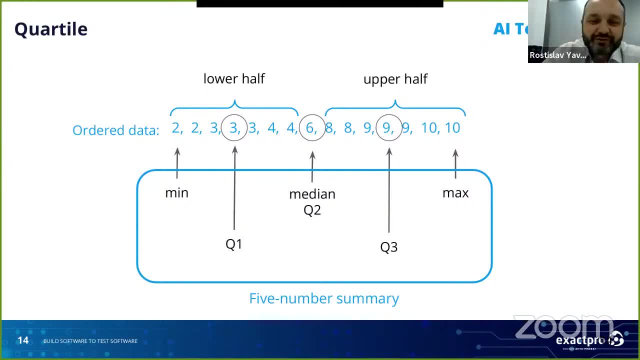 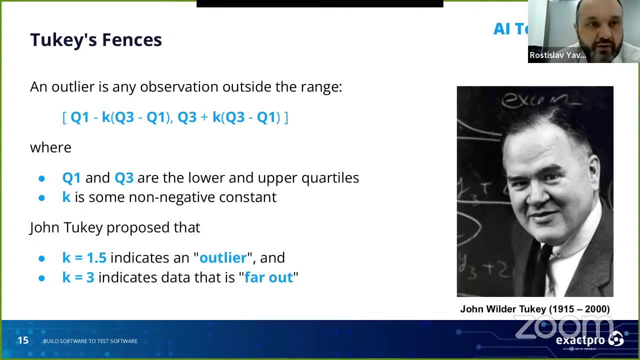 kind of the more informative way of short summary is called five number summary. So when you provide not only minimum, maximum and median value but also the quartiles. So, and this is this notion of quartile is the basic of very well-known Tukey-Fancy test. So, John Wilder, Tukey is a 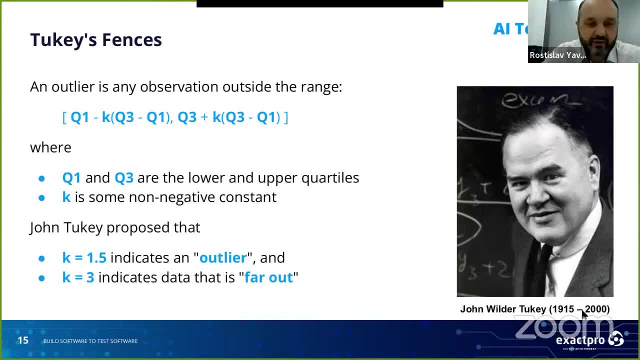 quite well-known mathematician. I just recommend you to read his biography on Wikipedia. You'll be impressed. So he's really a cool guy. So he suggested to use this again. quite simple, but why? it's useful? because it's completely automatic, So you don't need to visualize. 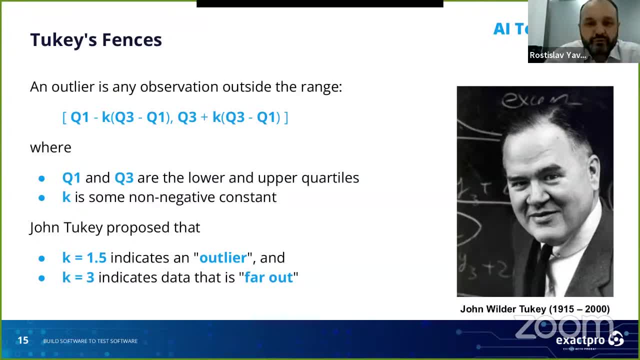 anything You need to look. you don't need to involve human to look at your pictures, at your scatterplot, at your histogram. So you just implement it and automatically you'll get a script which, okay, it says this is outlier and this is not. So the idea is quite simple. 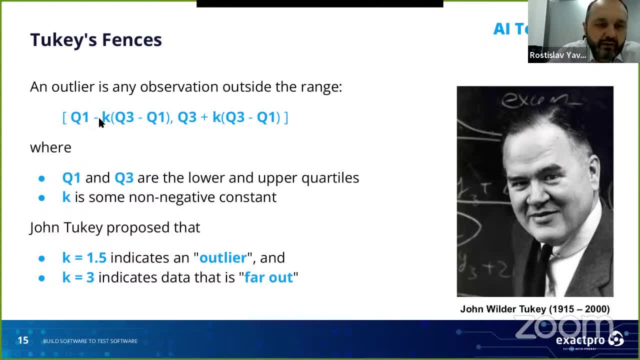 So you use the formula: just take Q1, first quartile, and then you minus some number of interquartile edge, where usually K is taken to be 1.5.. And again, this is magic number, but it's come from experience of many people. and similarly Q3. 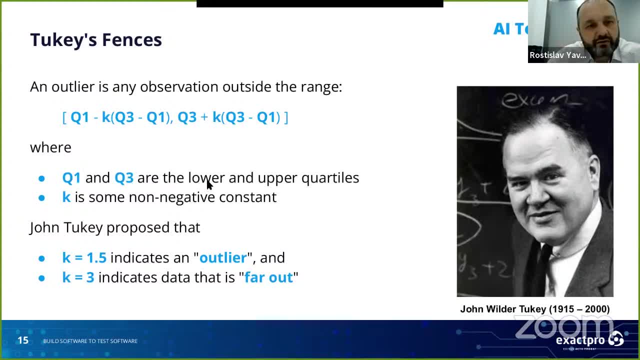 So Q1 and Q3- here are exactly the lower and upper quartiles which I just described, And K is some non-negative constant So you can play with it. maybe for your application you can take different value, but usually if you take K 1.5 and some data point falls, 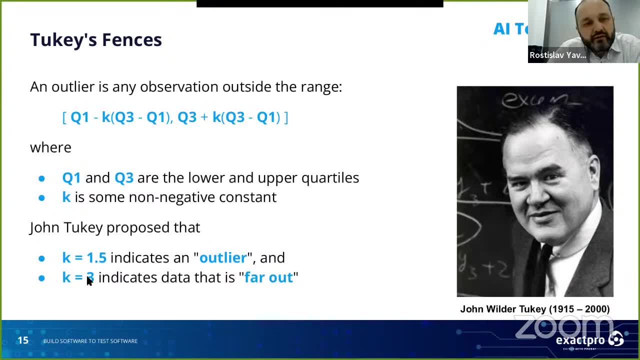 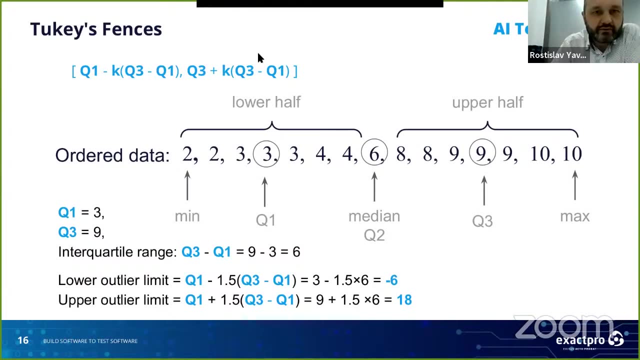 outside this interval, then definitely it's outlier. And if you take K equals 3 and some data point falls out of your range, then it's kind of far outlier. So let's see our example. So here's just the formula I copied here. So 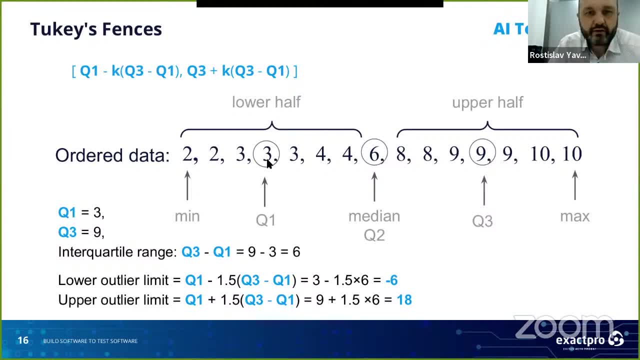 in our case, the first quartile is 3, right, It's here. Then the third quartile is 9, right? So the interquartile range is the difference between the third and the first quartile is 9,. 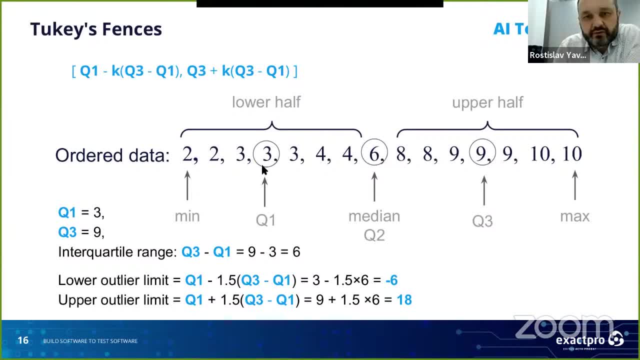 9 minus 3 is 6.. So 6 is some kind of the size of our core of the data. Then we just take Q1 minus 1.5, this size, So it will be 3 minus 1.5.. One point minus the number Six is a difference. 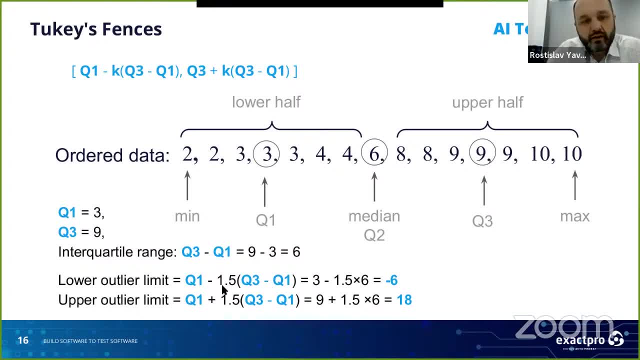 So it will be nine. 3 minus nine, it'll be minus 6.. And here I see this typo: it must be Q3 here, So Q3 plus. So yes, it's, it's here 9.. Q3 plus 1.5 times six, So it will be 9,5.. 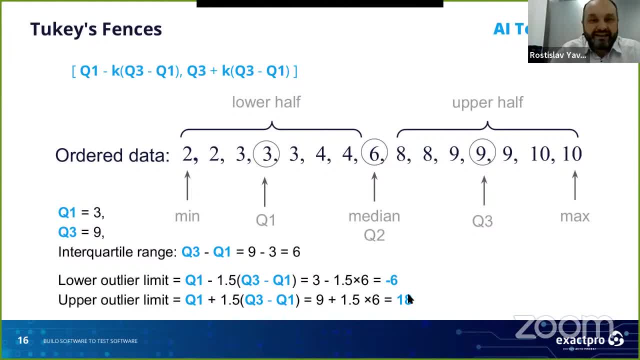 So what does it mean? So that if at some step you get data point which is below minus 6,, minus 6, so you see here just lowest point is 2, or something which is above 18, and see so far you have maximum 10,, then according to two preferences, these numbers will be outliers. 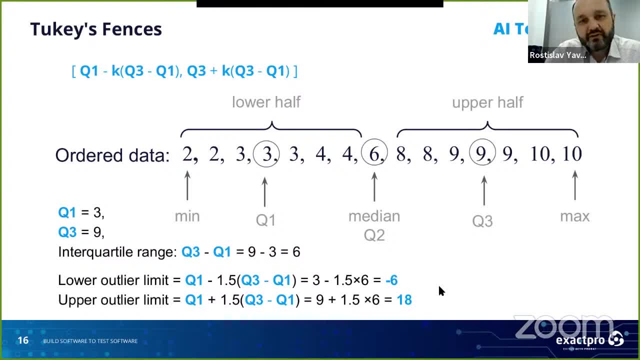 So, according to this test, you don't have outliers in this data set at all. So which I mean? even the smallest and the maximum, the largest values are not actually even candidates for outliers. And again, the main advantage of this data set is it's very simple, it's very easy to interpret and it could be implemented automatically with any specific knowledge of programming or mathematics. 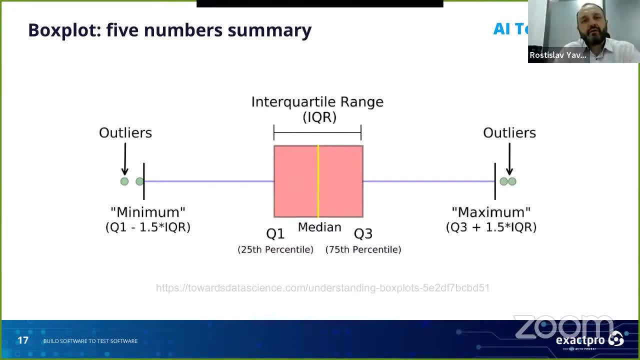 So, but again, this five-number summary could be visualized using this kind of diagram which is called box plot, And the idea is simple, right? So you indicate this interquartile range. it's colored here, it's kind of pink, so you can indicate minimum, maximum. 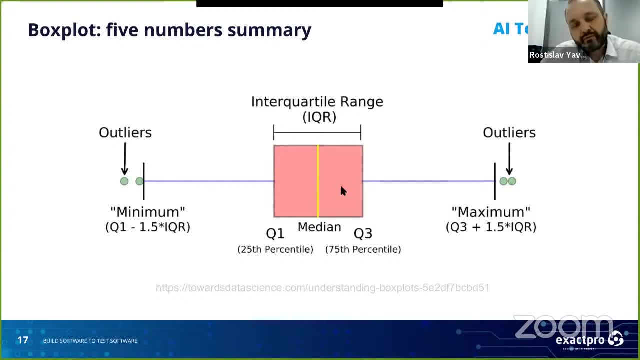 And sometimes you draw it for your data set, And sometimes you draw it for your data set And sometimes you draw it for your data set And sometimes you just remove outliers and then you draw this box plot and then you put the values for the outliers. 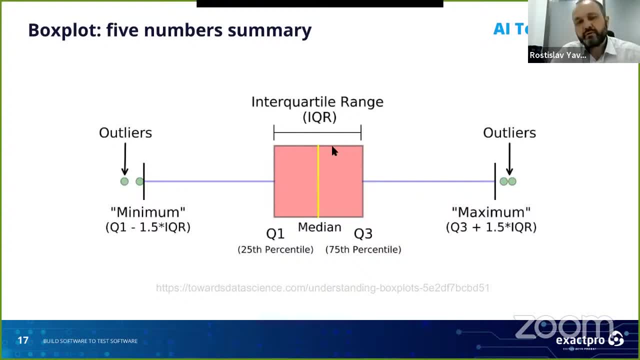 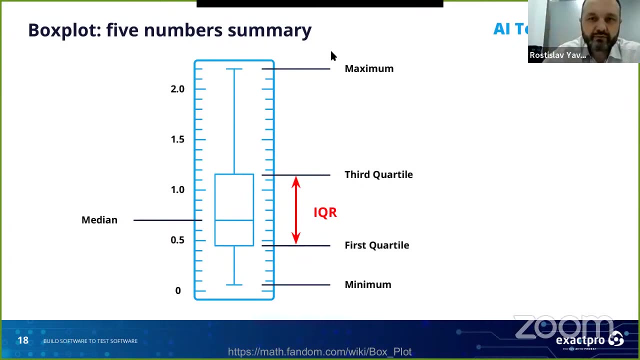 So this is a very useful, very simple, very widely accepted type of visualization: statistics of a box plot, And sometimes it's kind of written this way like maximum on the top, minimum on the bottom, And this first and third quartile are here. then median is indicated here. 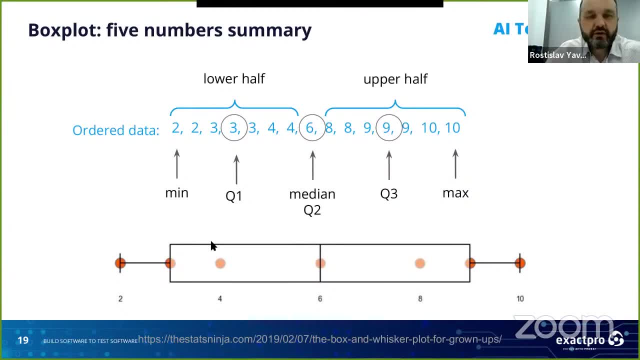 Sometimes- and this is exactly our example- sometimes you draw it horizontal way right Again. so minimum here is two, and first quartile is three. you see, Then four, six, eight are just our data points, and nine is here it's third quartile. 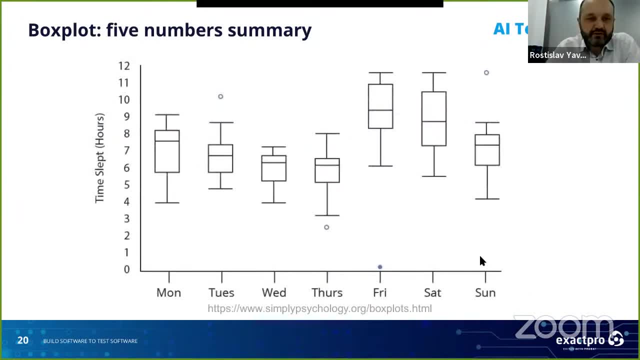 And maximum value. And this is just another example from more real life. And what's here? Ah, this is quite a funny example. So time slept hours here and here. you have like seven days of the week, So assume you just had some survey in your office to check how much time do people sleep? I mean every particular day. 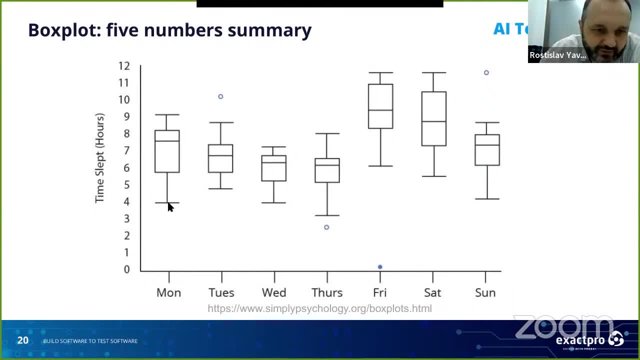 So let's see the Monday. So you have, there is a minimum value. So there is a person in your office who slept just four hours, but there is another lucky guy who had like nine. But you see, the median value is something like 7.7, and third quartile is around eight. 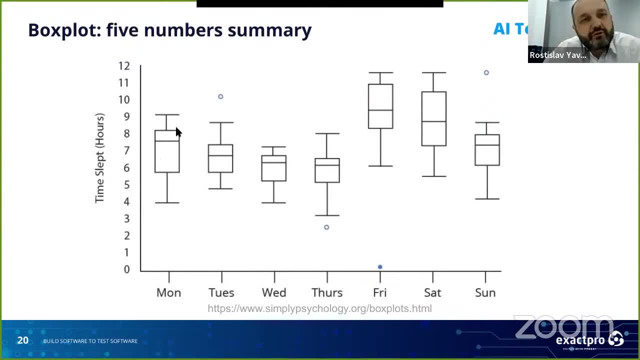 First quartile is something like around six. So you see, the majority of your- like half of your friends, colleagues just sleep between six and eight hours, but there are some kind of minimum maximum value. So let's see, Tuesday- And this is the average kind of- is below, slightly low than Monday. 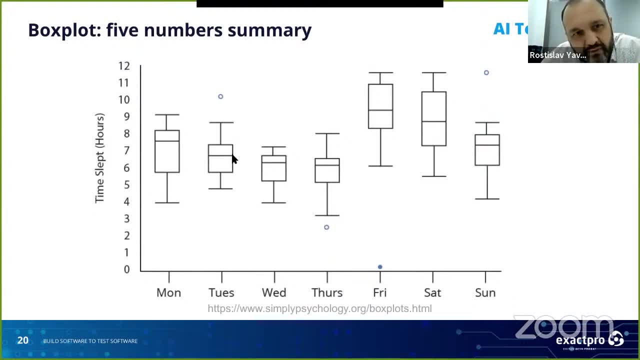 So the median is just below seven, But you see the minimum is more. So probably this guy had the party during the weekend But no, no party on monday. so at least five hours is the minimum, and this is somewhat liar. there's a lucky. 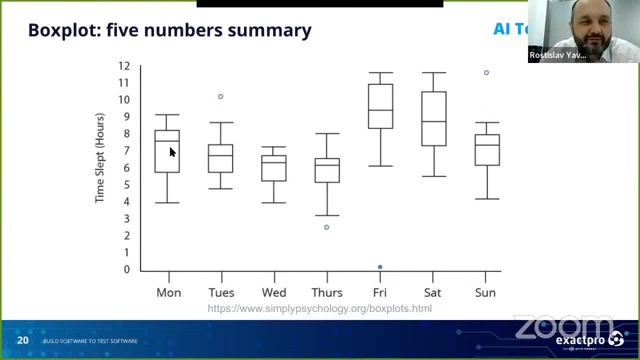 guy. probably he or she had some deadline on monday so it was kind of lucky. or maybe his vacation starts on tuesday so he spent in bed almost 11 hours. or maybe this is just this guy who had a party on monday. then you cannot just have two parties sequence, so he decided to just 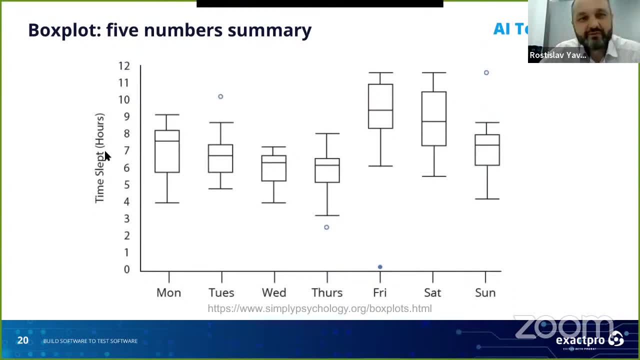 took day off after just completing urgent task on monday, so you have here like more than 10 hours. so you have wednesday, which is again average, even smaller than tuesday, and thursday is is even below, but friday becomes much, much better. so you see, even the minimum is six. but 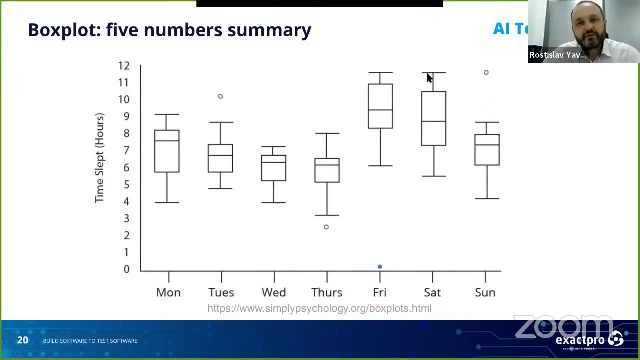 first quartile starts about eight. so you see, so you have five numbers summary for each of the day. so you put it, put them on just one, one screen and you have quite, uh, quite good understanding of what's going on with this parameter again. so you have visualization of just one parameter, just one single parameter. 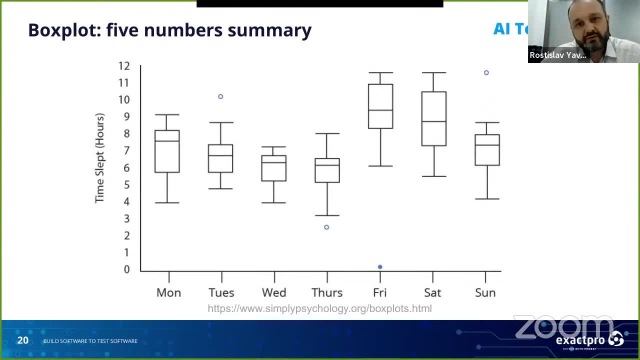 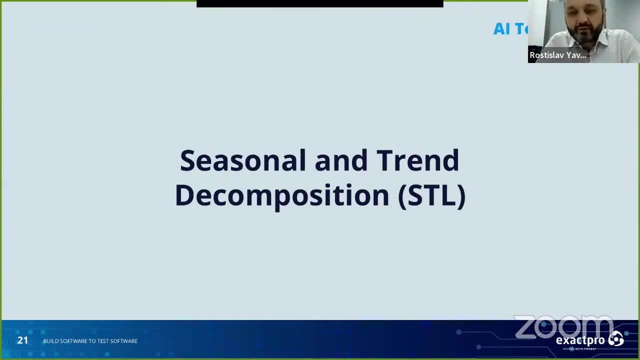 times left in hours. but anyway, this is, this is quite, uh, useful and very informative. so that was quite simple part. okay, let's gradually, gradually, move to more advanced technique, and now we will speak about time series. so you have, for example, some measurement which goes over time. oh, probably that was just a good. 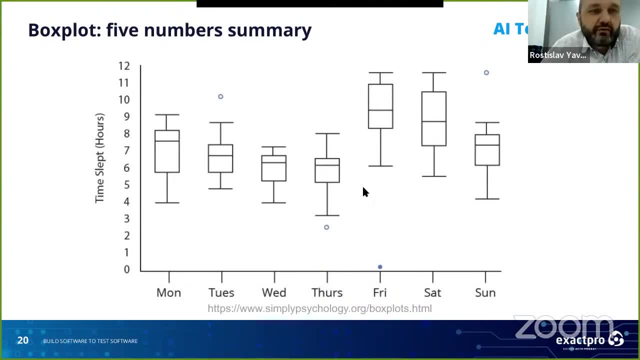 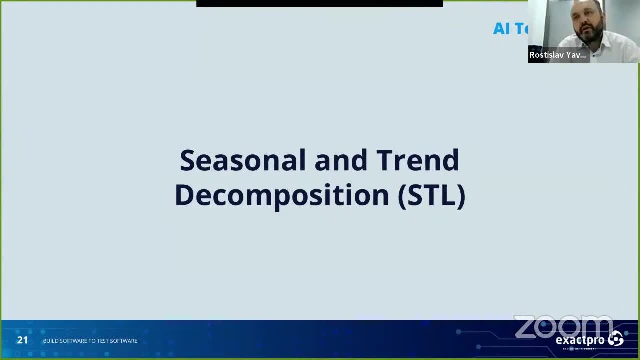 example of time series. so you have a value you measure daily or, for example, it could be measured hourly or monthly or every second, or doesn't matter. so you have some time series and you need to figure out some anomaly in this series. and then one, still simple but power technical, is called seasonal and trend. 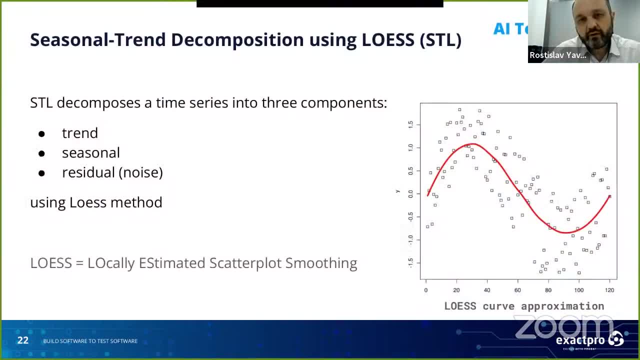 decomposition, which is the abbreviation, is stl, and the idea is, for those who of you who know what's linear regression and linear approximation, this is kind of generalization of a generalized version of a linear approximation for for more advanced trends which could be not linear. so the idea that your algorithm decomposes a time series into 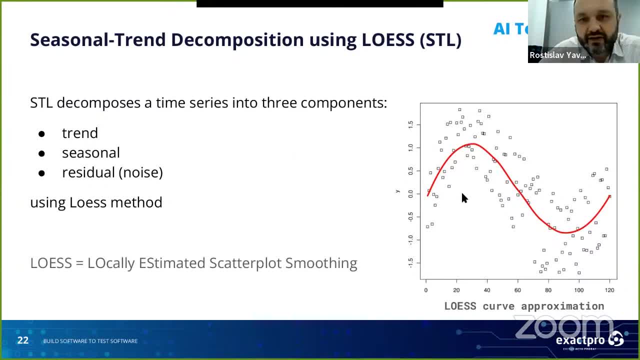 three components. the first one is called trend- it's uh, it is uh, red on this picture. the second one is called seasonal and then the remaining part is called noise. so this already um uses some advanced mathematical techniques, which is called loss from locally estimated scatterplot smoothing. and okay for this technique. 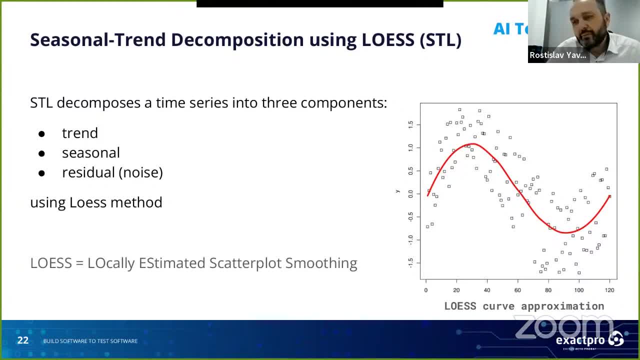 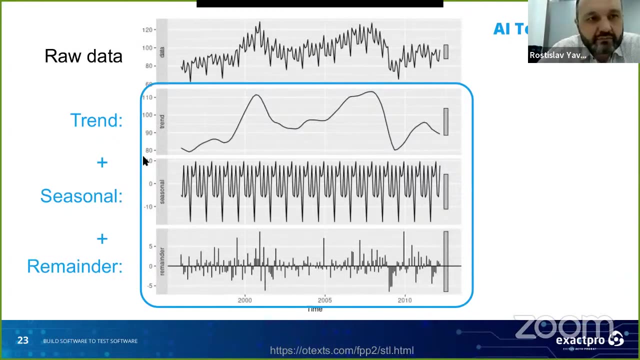 you probably would not like to implement it yourself, i would suggest just take out of shell some maybe standard library or whatever. so there are a lot of different implementations on the web. so but basically the idea that you have some kind of raw data. so you see, it's on the picture above. 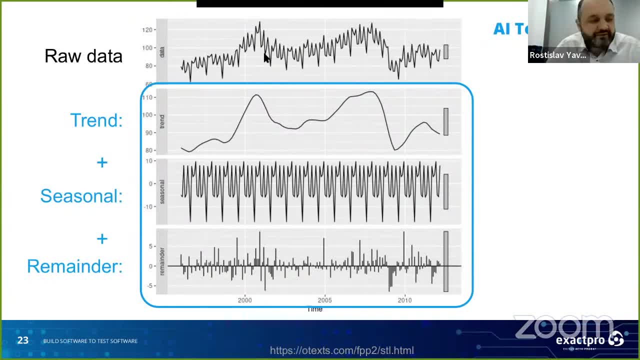 and you assume that, okay, this is your basic assumption of this method, that it could be decomposed into three components. first, you compute trend, which could be any kind of like- uh, this kind of curve. so, for example, you have some sales, or like traffic on your web or whatever. so you assume 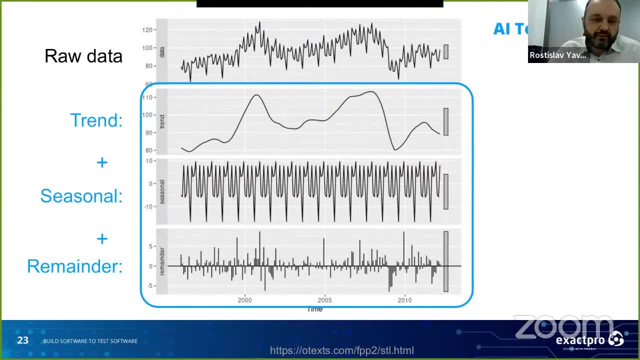 that traffic couldn't be the same like yesterday because, for example, it's different season, like your investment, something in your marketing, marketing campaign and etc. etc. so you have some trend in your data and also you may have some seasonal components, for example, if you have some weekly data always. 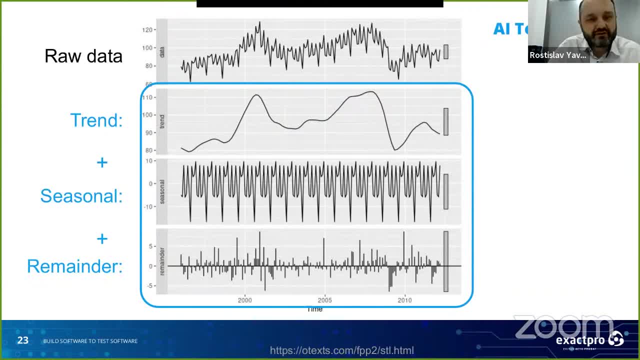 you will have something different during weekends and during working days, so you have something which is a behavioral relates on the date of the week, for example, uh, and then the remainder part. so let me remind you that our topic is anomaly detection for ai testing, and i assume you 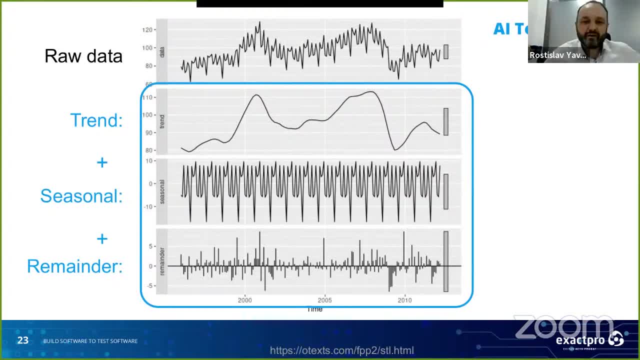 already understand the basic idea that in order to define, to find out anomalies, you first need to define what. what is normal? and in this approach, your assumption that normal is combination of trend and seasonal uh values. so you see that, okay, we assume that this seasonal graph is is kind of normal behavior and this trend is okay, it is explainable, kind of part of your. 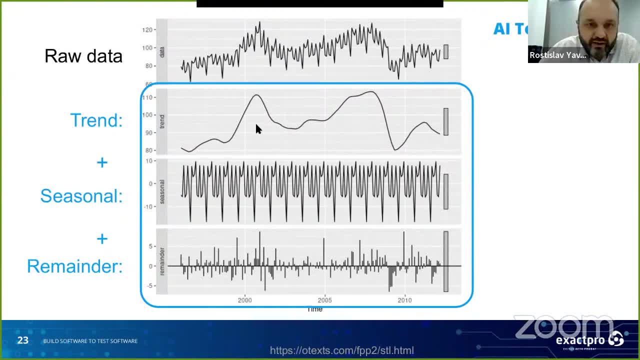 data so and then you just try to find out kind of the best approximation of this tool, and then the remaining part, the reminder, is located here, so you don't need to look at points here, but instead you try to to analyze reminder in order to find your anomalies and outliers. So you see like here and 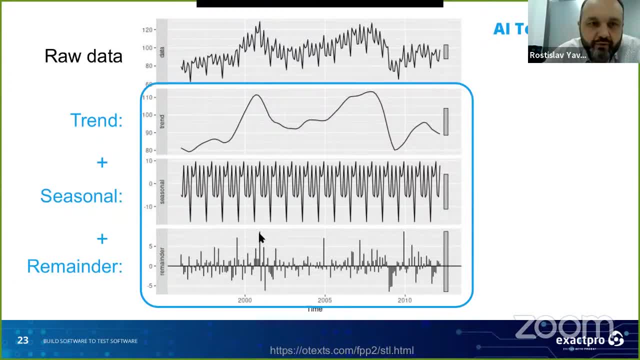 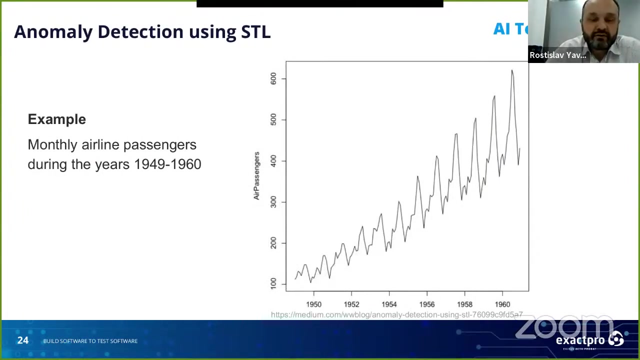 here you see some really deviation from your trend and seasonal behavior. This could be a candidate for anomaly, this is another one, and this another one, etc. So you see, basically this is quite useful and powerful method And there are quite many good texts on the web about this method. I 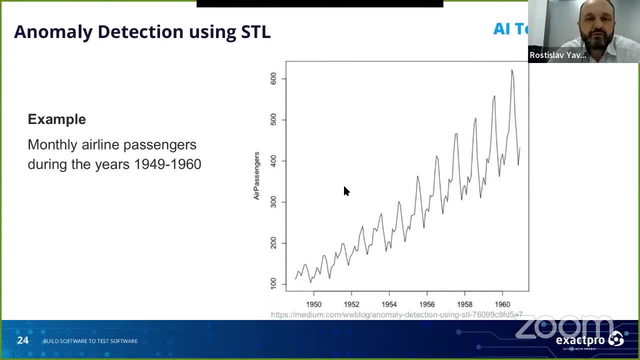 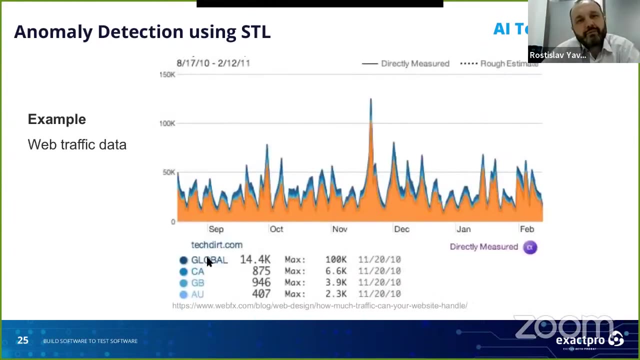 really recommend you this paper on MEDIUM, which is about anomaly detection using STL from monthly airline passengers data. So the link is here and you can easily find it, And another good example for applying STL is Web2.. So this kind of data each of you can easily access by installing Google Analytics or 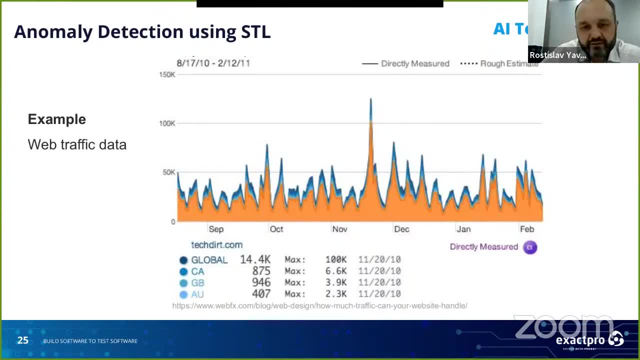 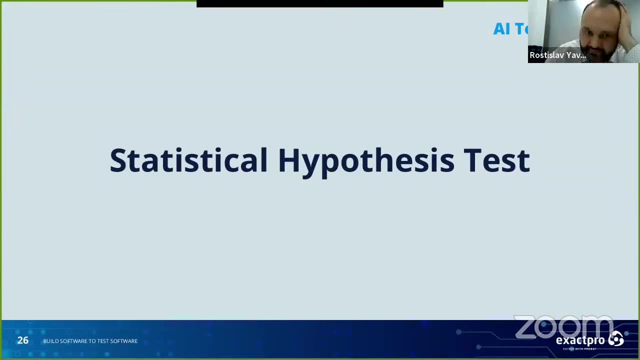 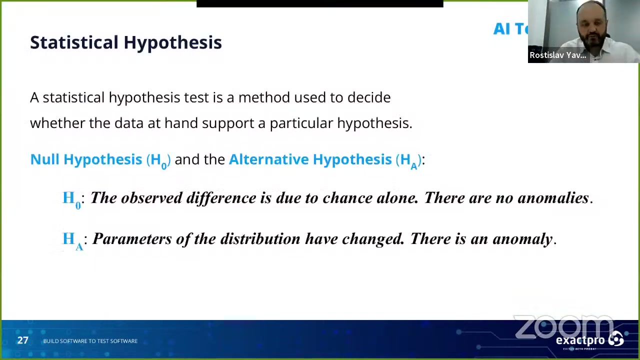 just any other statistical analysis for your web page, So this data could be very well analyzed using this method. Okay, still have some time. Let me switch to the final section of our today lecture. It's about statistical hypothesis test. So the idea is that for statistical methods, 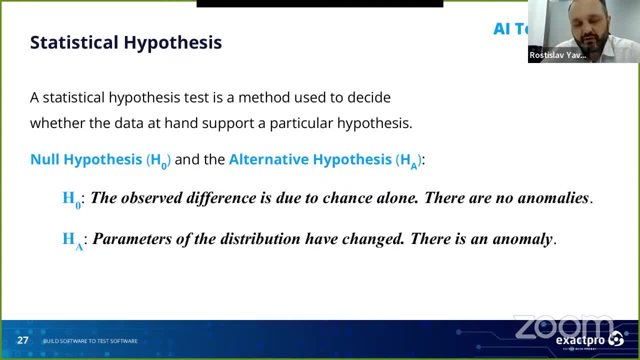 working is hypothesis and parameters is kind of quite a well-known technique. So this task to check whether some hypothesis is correct or not was well studied during the 20th century, So a lot of quite powerful and interesting methods were developed. Let me just give you a short introduction into 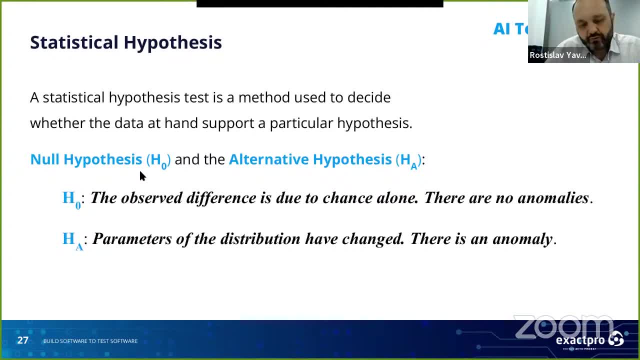 this topic. So usually to use this method you need two hypotheses: The one which is called null hypothesis. It assumes that kind of everything is stable. It's stable like we have normal behavior. So the observed difference is due to change alone. change alone and there are no anomalies. So this 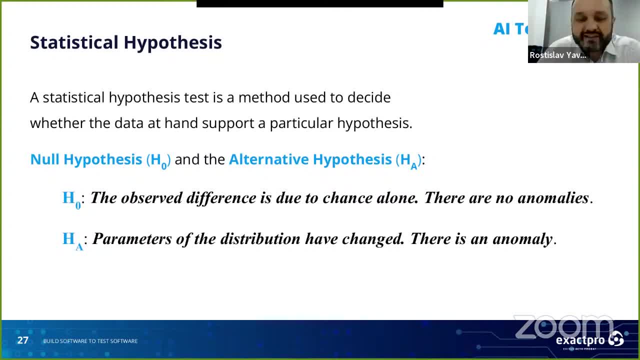 is just a general scenario. There are no LGDs and other things that the data can be used to to do anything, So definitely. we are working with random variables, So you cannot have the same data today as you have yesterday or the day before yesterday, but all changes you have are just due to. 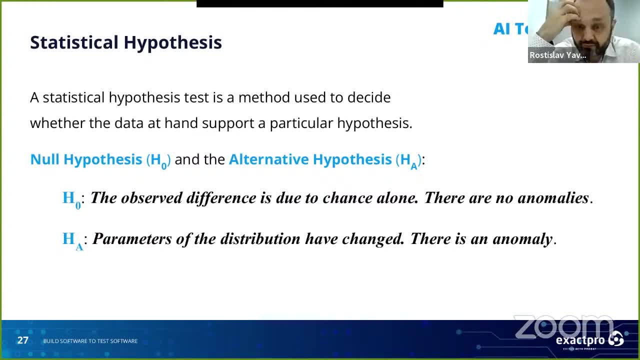 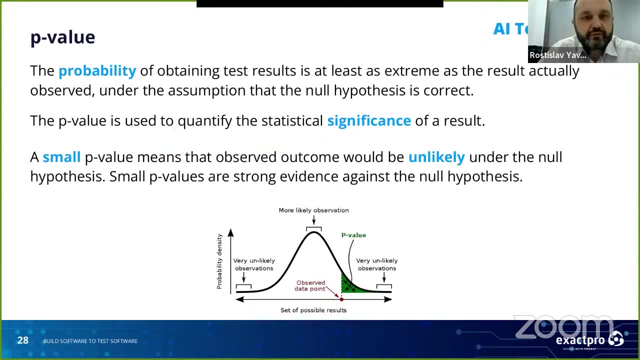 chance alone. And then you have the second hypothesis, which is called alternative hypothesis. It has the parameters of the distribution have changed. So actually you have anomaly and the data tools have to measure how this second or first hypothesis is kind of true. so the first very 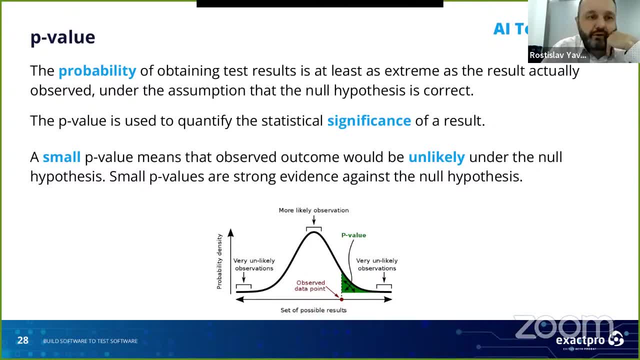 important characteristics of your data is called p-value. so- and it's really important- that's probably the basic, the most important notion in this area. it's widely used by statisticians and in different applications. so what's really p-value? so p-value is the probability of obtaining test. 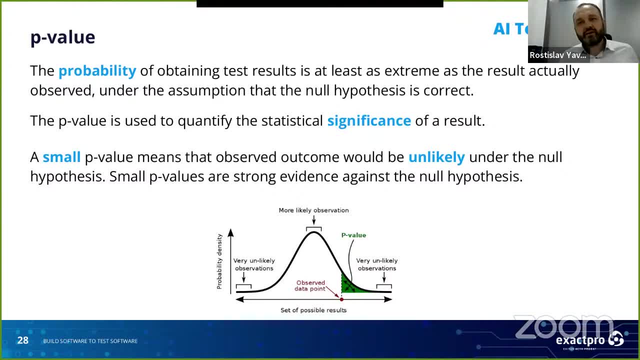 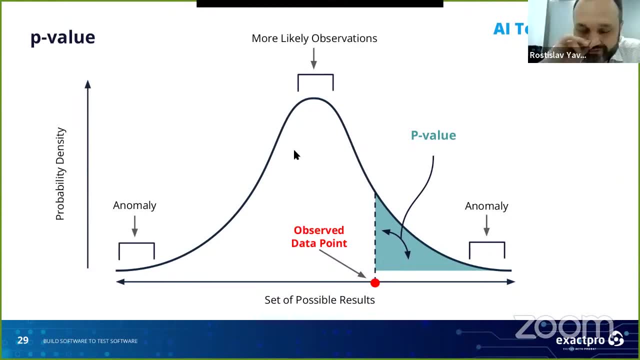 results which are at least as extreme as result which you got. so let's look at this picture. so assume you have quite okay, you almost never have seen application so, but so okay, let's assume you have a very nice symmetric picture of your distribution. but p-value surely works for any. 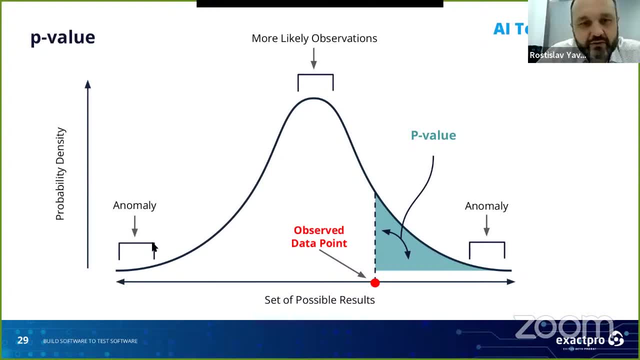 kind of distribution, but at least for this example, let's assume you have this nice curve, so this is a probability of the distribution of p-value, of the distribution of p-value, of the distribution of vips, where your distribution values are. you actually have very high probability of different. 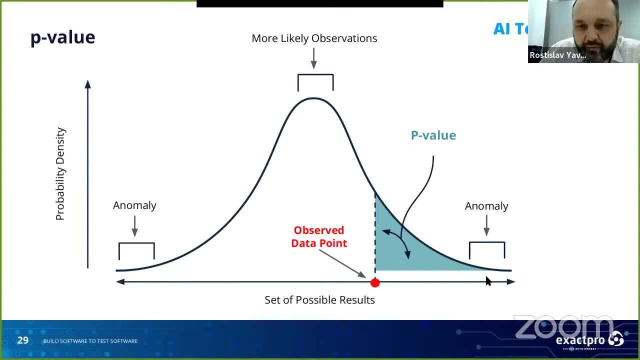 values. so the total area below the score is equal, equals to one because to 100 percent. so this is kind of all possible values. so here you have kind of peak of your distribution. so more likely observations are located here and so you expect some values around here which account here and 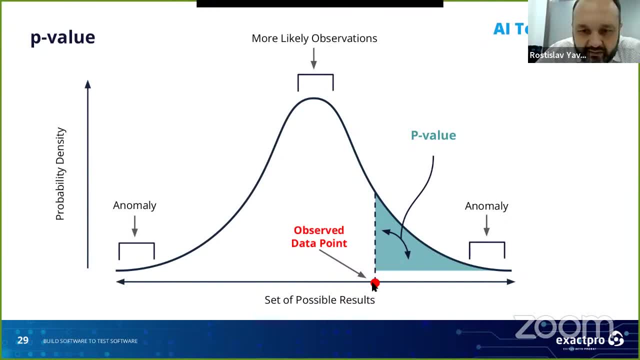 then you perform your measurements and you get this data point. so this is the observed data point and you realize: okay, load data is g color over. it's going to be so. point abs et al, equals year, not really among the most likely, but it's not actually look like anomaly, so it would be really. 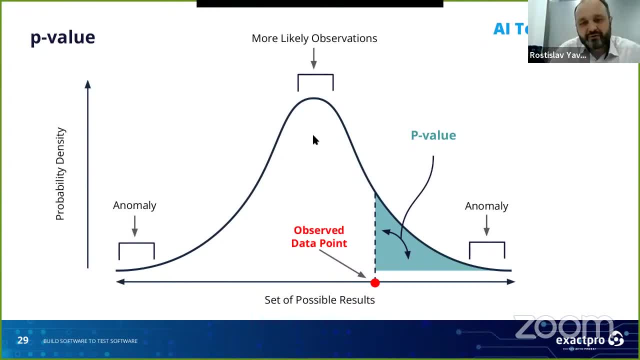 nice to have some tool how to measure your feeling, because again, once you, uh, each time you, you need to to do it manually, to do it like with your observation, with your kind of a visual you to apply visual possessions. it takes you time, so you would really prefer to have some automatic test. 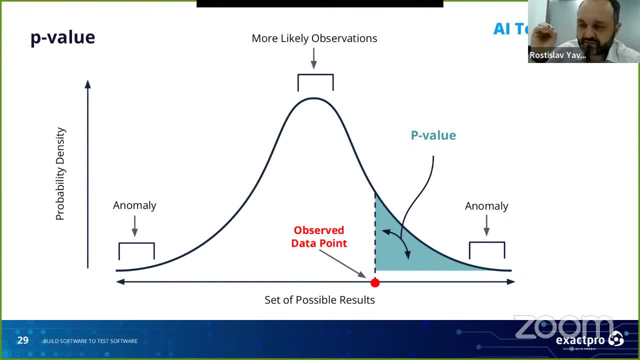 we just compute some value, apply some test, and then it says, okay, this is just anomaly, one, normally two. and this is number three, just another candidate which you should consider maybe or not, but uh, okay, so p value is exactly the technique to measure the measure. how far is uh your observed? 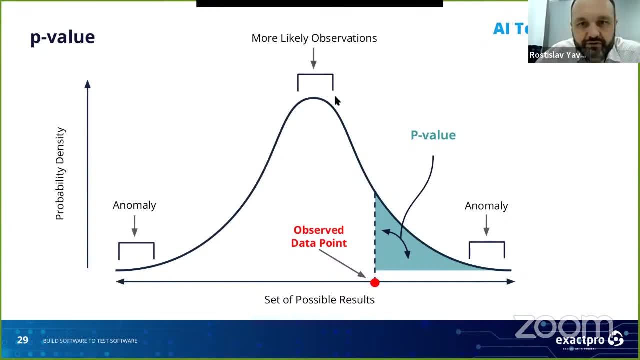 data point from more like observation, and the idea is that p value is the error below this curve, which is kind of uh about this value. so you got this result, for example, like 22 or 25- uh doesn't matter- and but still it's possible to have 26, 27, 29 like, even maybe 40 is still possible. 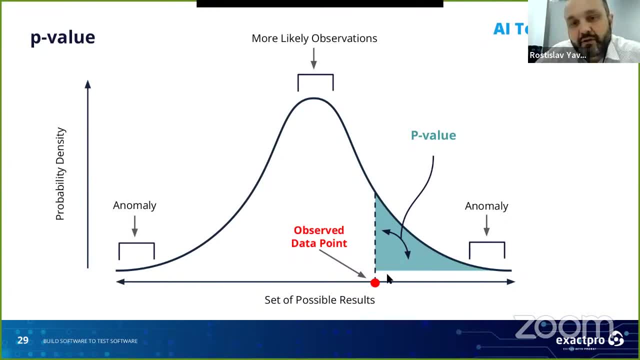 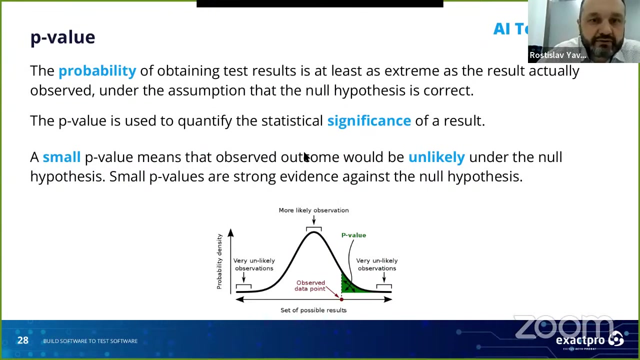 according to your distribution. but the probability of this of these values is really small. so in order to measure, to measure the probability of your alternative hypothesis, you compute the sum of all probabilities which are about above your observation. so actually, p value is just used to quantify the statistical significance of your result. so if p value is small, 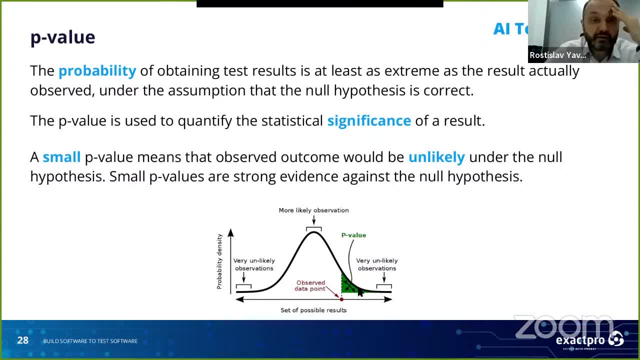 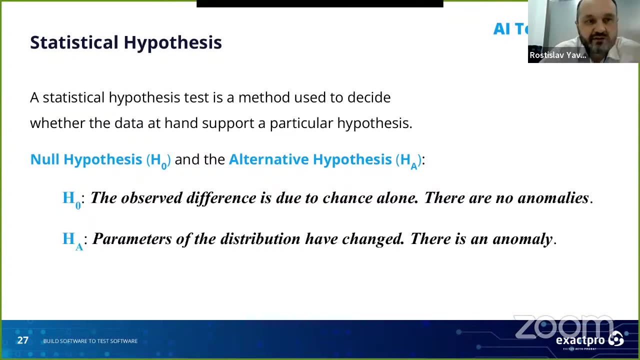 so if this area is small, that means that the probability of your kind of that everything goes well is quite, quite low. so that means that your outcome is really unlikely under the null hypothesis that everyone, everything goes okay. so if you have very small p value, then most probably 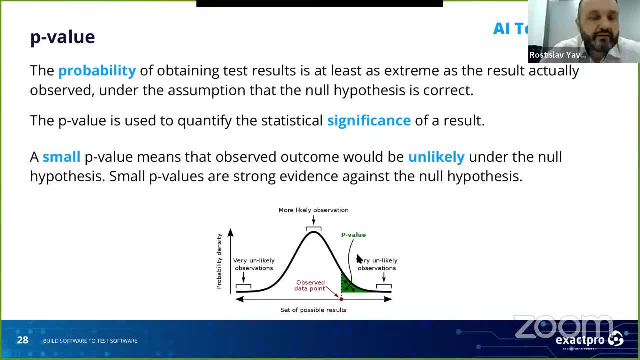 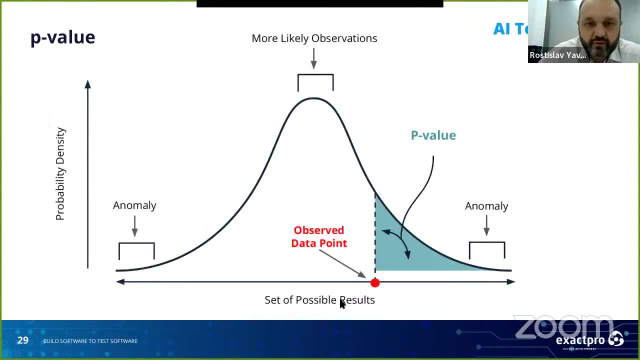 you have anomaly? and if you're, let's consider another example. for example, you computed some, some observed, you observed some data point and, uh, you had a feeling, right, okay, that's probably an anomaly. but then you compute p value and it turns out that p value sounds like like 50 percent. okay, not 50, even 20 percent is. 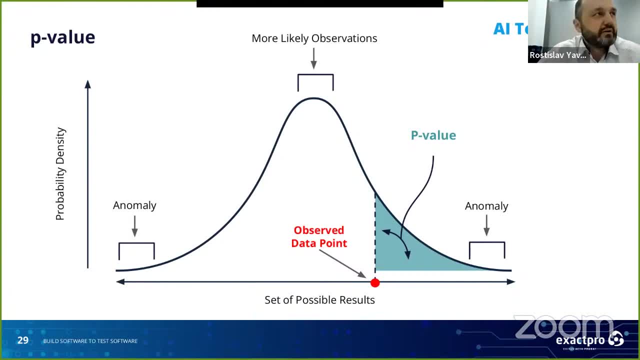 quite big value. so usually it's considered like anomaly if it's less than five percent. so 20 chance you observed, you can observe something even far from more likely observation. then this p value 20 percent, you'll say no, they think it's not like. uh, normally that's just another. 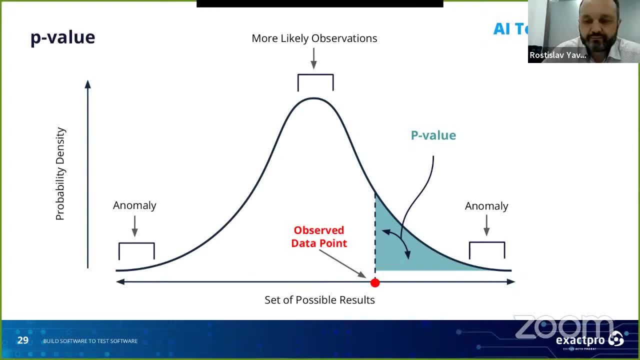 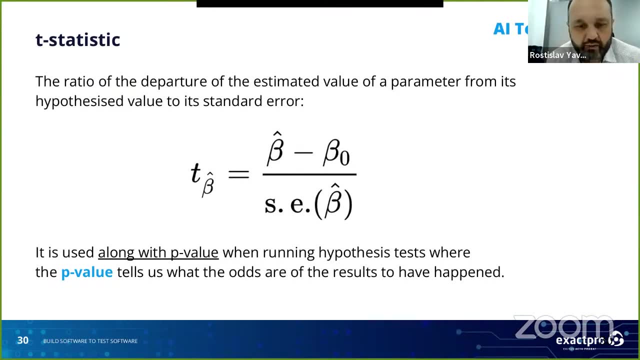 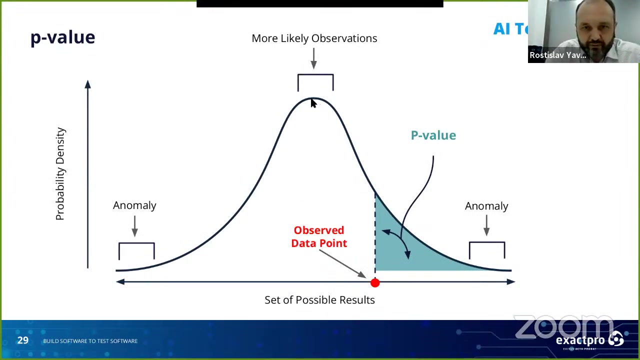 okay, that's because of your random nature of your, of your data. so, and another, another parameter which quite usually used is called t statistics, and here is another simple formula. so you have estimated value, you have your hypothesis, and then you just normalize this difference with your standard error. so let's see this picture again. for example, your expect value here is like: 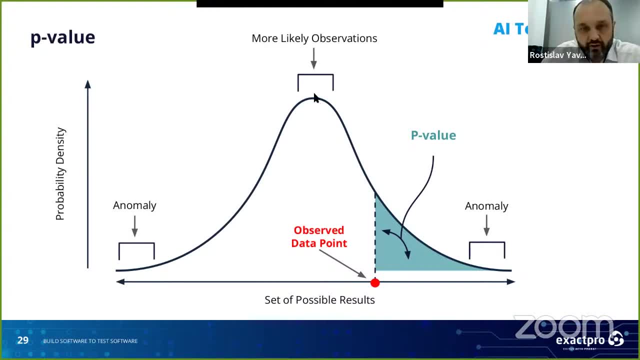 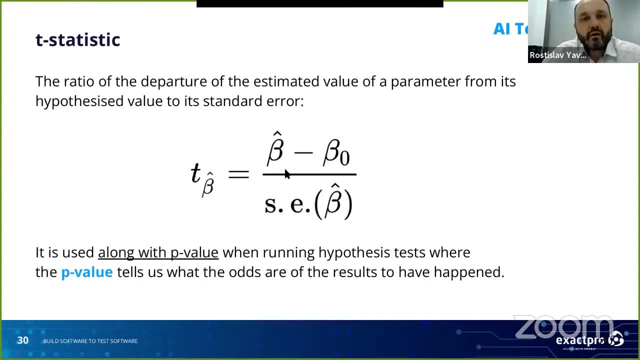 okay, let me say 22 and then you observe 25. so here estimated value is 22, observed value is 25.. so you say, you see, our observation differs from our prediction, like the difference is three. but again it may, sometimes three is something small, sometimes three is one something. 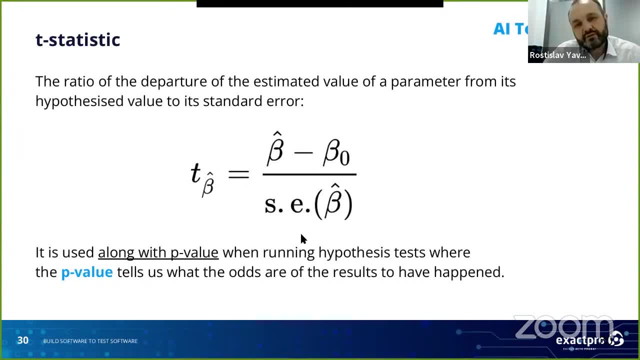 big so you need to normalize it with standard error. so the send the immediate question is okay, and what's the standard error of your data? and if standard error is like uh six, then you say okay, then three divided by six is like just uh 0.5. so difference is not that big. so if your 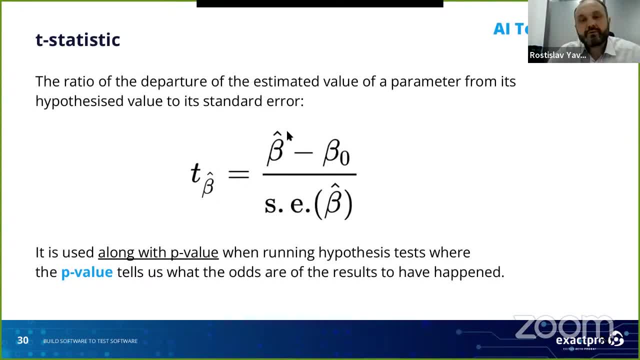 standard error is rather small. so typically, typically, you have like observation 22 and standard error is below than one. then observing 25 is different story. uh, so you see, and uh, okay. so that means that uh 25 in this case will be, will be quite a candidate for anomaly, and this t statistic is usually used along this p. 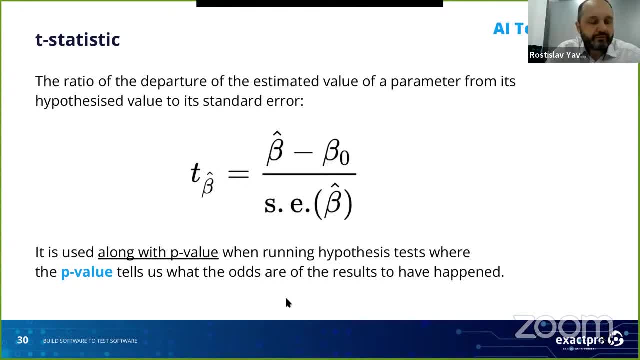 value. so typically you, you come to your okay boss, your manager, say you see, you have observed value like 25 and it's quite far from our prediction and the p value is rather small, so, for example, less than five percent. so the chances that this is uh just due to our kind of standard, uh kind of 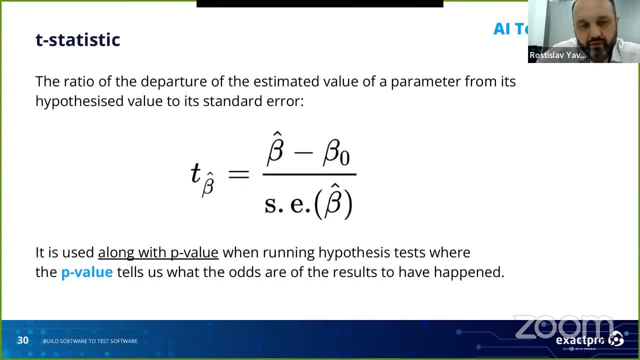 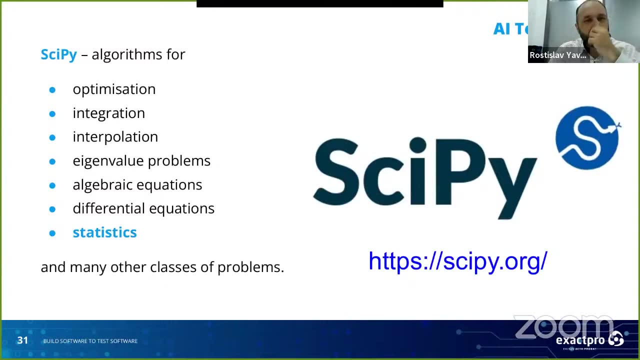 random error is is very low, so most probably this observation is anomaly, is outlier, so let's analyze. so this is actually all i have for today and before i mentioned. some of the techniques could be easily implemented manually, like computing, computing quartiles, interquartile range or 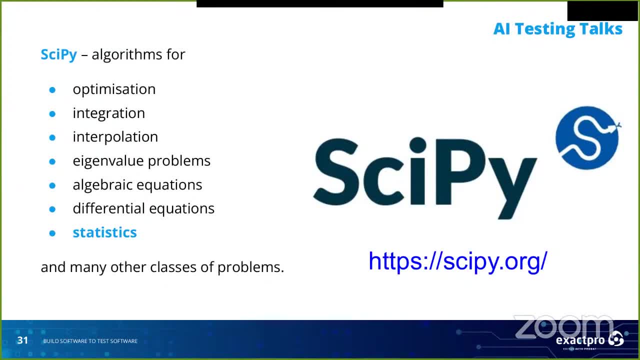 this five number summary. but the more we kind of go deeper into statistics and dive into different methods, you definitely would prefer to use some library- and here just link to very kind of popular, powerful and famous library which is called scipy, which includes- definitely includes- different statistics, uh, but also a lot of algorithms for optimization integration. 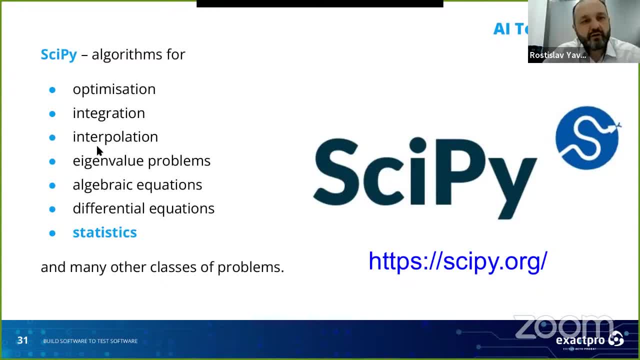 algebraic equations, differential equations and taking value problems. next lecture we will speak about machine learning approach to anomaly detection and this will be also useful here. so for different methods and many other classes of problems, but i will try to explain it in a few minutes. So definitely for more advanced techniques. 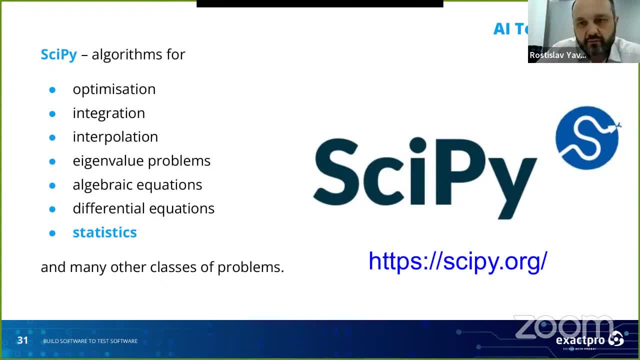 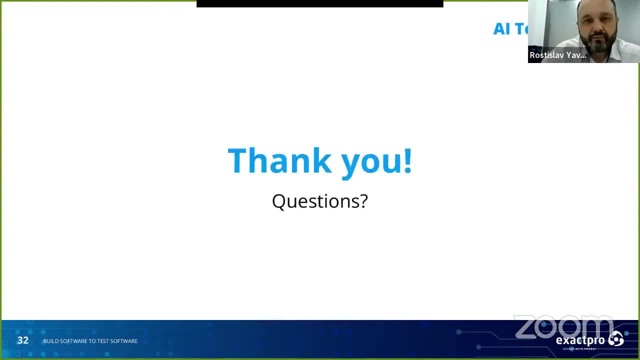 you don't need to do it manually yourself. You can use different libraries. it's just one of them, And surely there are different options too. So thank you again, And questions are welcome. So most probably we'll have a separate session for questions answered. 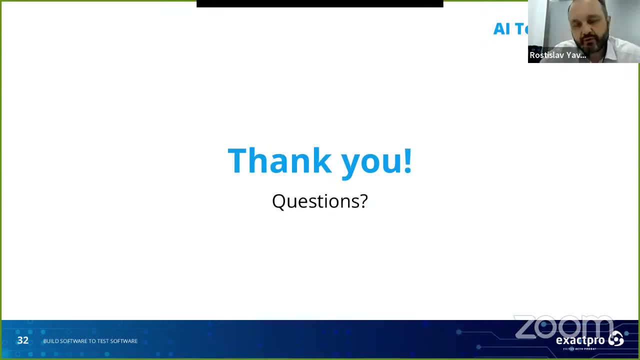 Just if you're looking at the recording, watching the recording, just put them in the comments And I hope I will have chance to answer you. So we still have one more lecture in this mini course. Like I said, it will be about machine learning approach. 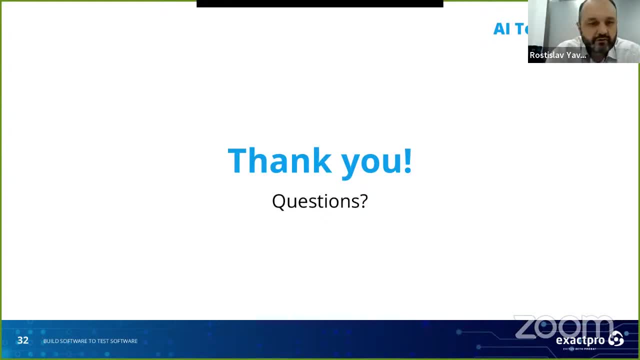 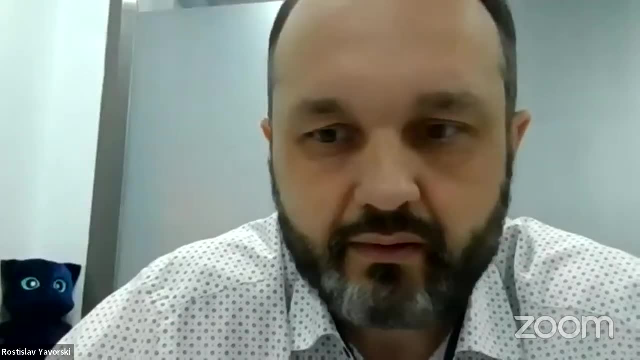 to anomaly detection, Most probably next week. just to see the announcement. Thank you very much. See you Okay.